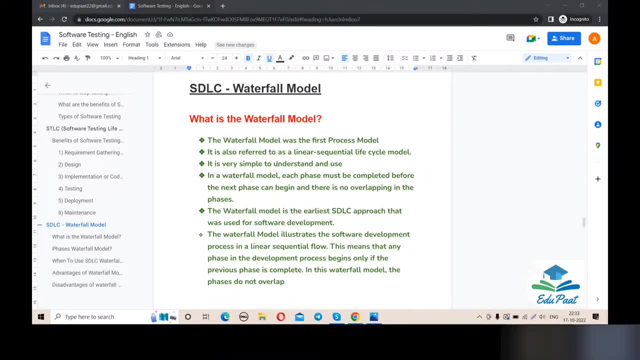 So hello guys, welcome back. So as a part of this video, I am going to tell you what is HDLC waterfall model. So, before we do the last video, I have already talked about what is the HDLC life cycle model and what are the phases are there And there are a few models we have discussed. 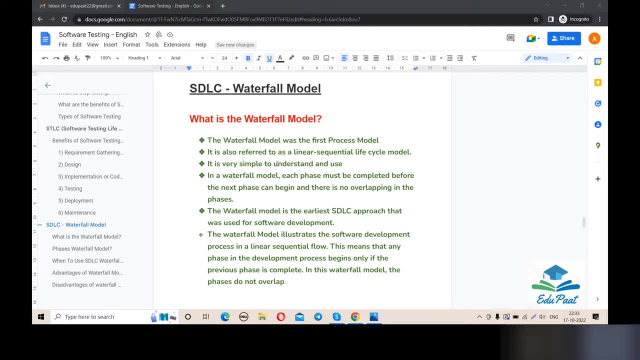 about the last video. like waterfall model, spiral model, then VNV model, then agile model, then prototype model, etc. etc. So today video I am going to tell you what is waterfall model in HDLC model. So let us talk about what is the waterfall model. So the name says that: the model. 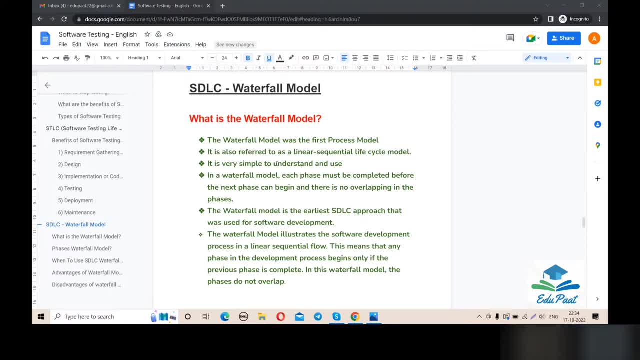 is looks like a waterfall, So that is why this model name is waterfall model. So I am going to see one phase structure, one model structure so that you guys can very easy to understand that how the names come as a waterfall model. Before that I am just telling. 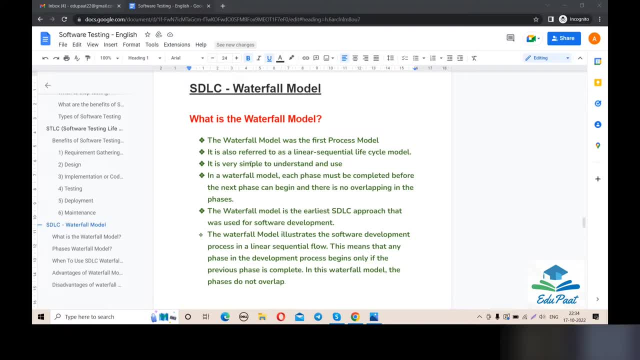 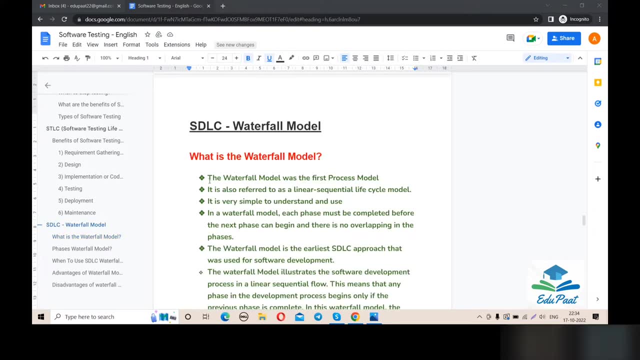 you what is the waterfall model. So I have documented few things as you guys. it will really helpful to you. So the waterfall model was the first process model. Waterfall model is the first process model. So in the software development. 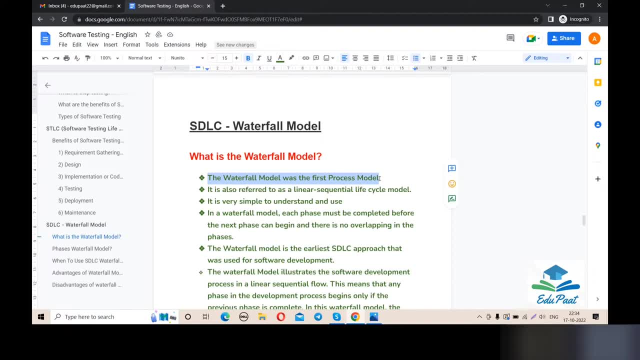 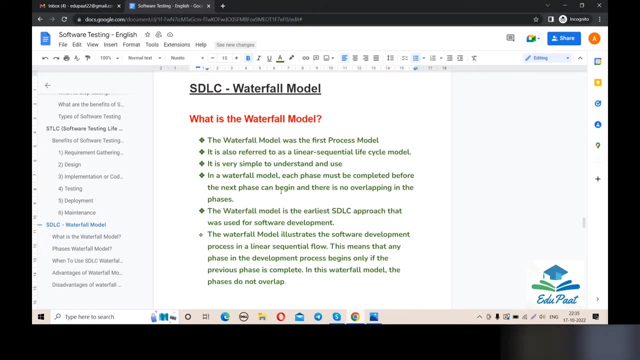 life cycle or HDLC model. the waterfall model is the first model. It is also referred to as a linear sequential life cycle model. Why the name comes up linear sequential life cycle model? Because in the waterfall model phase in the development process, 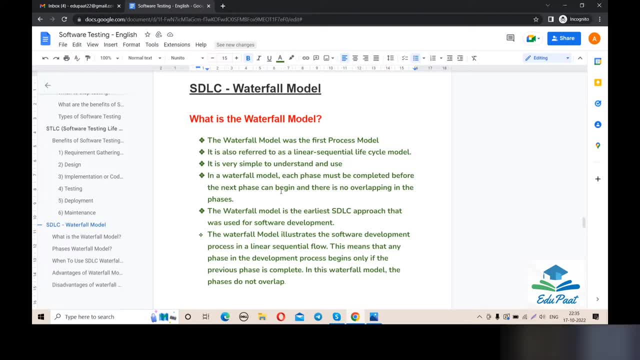 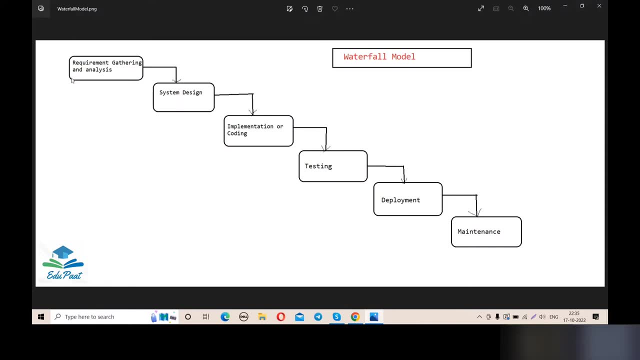 the previous phase is complete. That means now I am going to show you few stages of waterfall model. So this is the waterfall model. In the waterfall model we can see that there are few stages, as there like requirement gathering and analysis, system design, implementation. 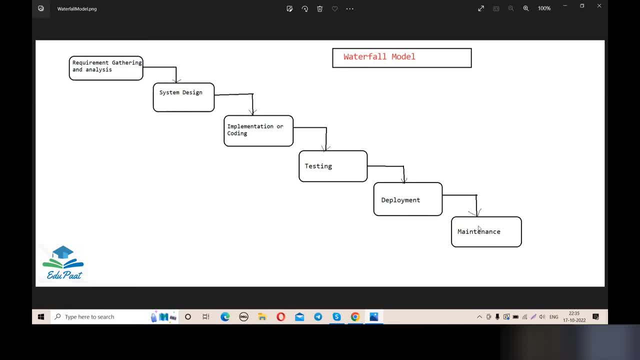 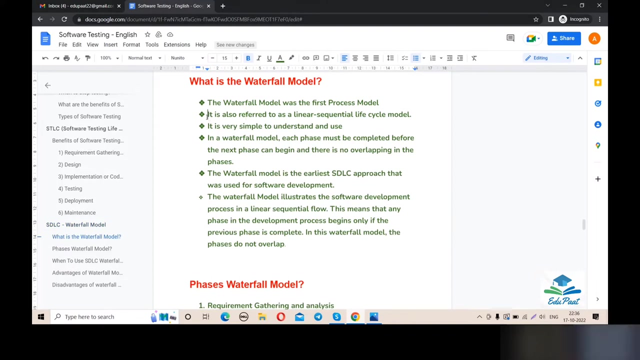 or coding, testing, then deployment and then maintenance. So there are six phases. are there in the waterfall model And, guys, I already told you that waterfall model is the ATX operator, That means underwater resources, is NFL JAMES THURSTON, BRYANT AND UP FOR compareRING FACTORS. In the waterfall model phase, you are going to see that the Department of Water没現 Waterfall Models- there are figures that are jed smashed come down to. the NEM is waterfall model. First thing is that. what are you doing with the name came waterfall model? Why the name is waterfall? 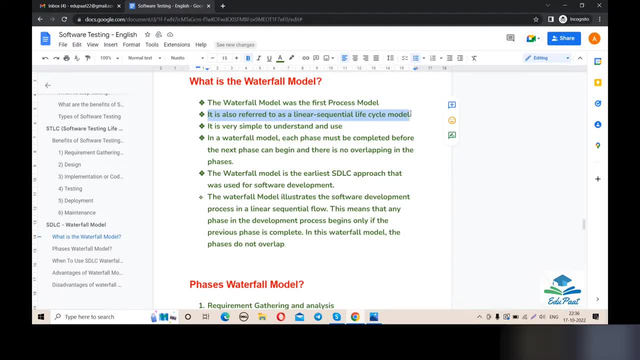 which is waterfall model Because, as you guys can see, that all the phases are showing the 달�ual to as a linear sequential life cycle model. then the third point is that it is very simple to understand and use as a waterfall model. is very simple and very easy to understand. why i'll tell. 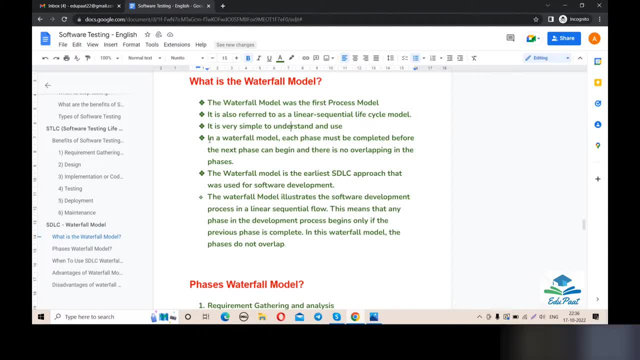 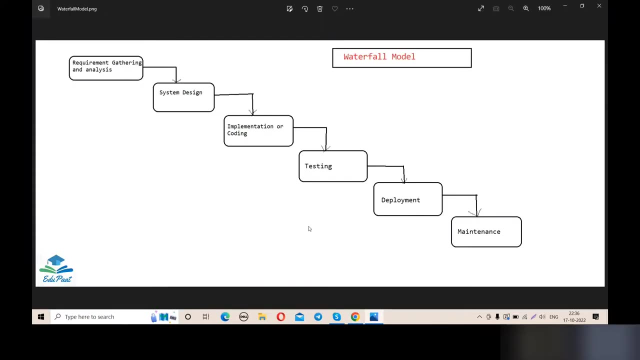 you later then the fourth point is saying that in waterfall model each phase must be completed before the next phase can begin and there is no overlapping in the phases. means this is the waterfall model. suppose i am on the testing phase. let's say i'm on the testing field. if i am on the 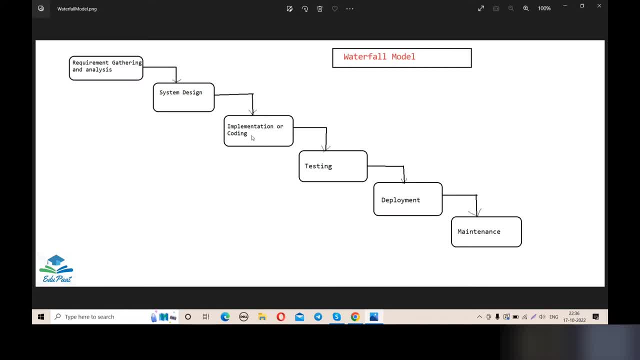 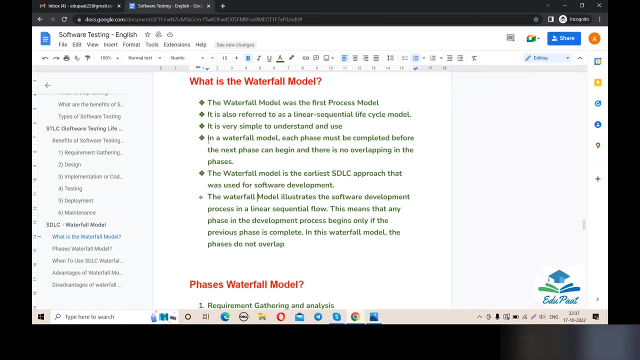 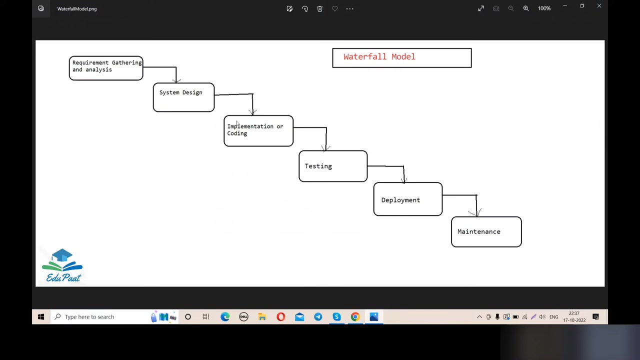 testing phase. that means we can tell that already implementation or coding phase done. right, so when i am on the testing page i cannot revert back to the implementation or coding phase. okay, that's why it's saying that in the waterfall model each page must be completed before the next phase. that means one phase will be complete, then the 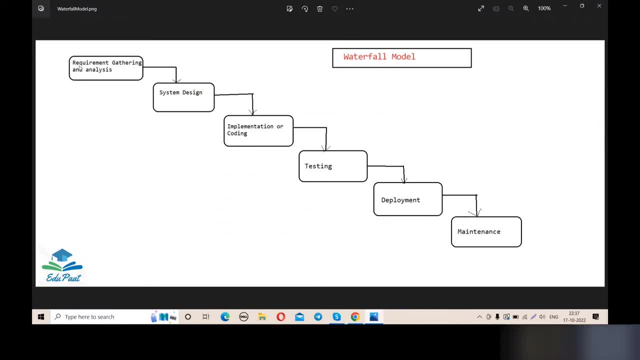 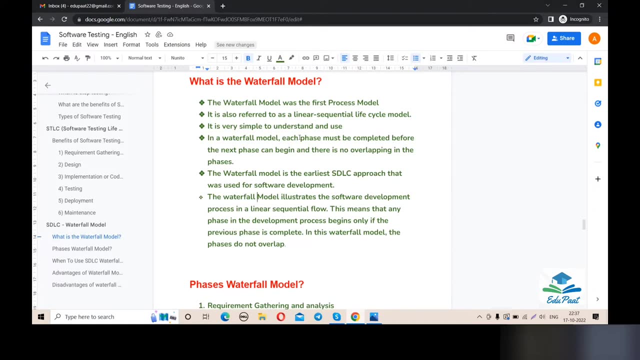 next. next phase will be start when the requirement gathering on analysis phase will be complete. then the system design will be start. so that is the process, like in waterfall model. so that's why i am saying that in waterfall model each phase must be completed before the next phase can begin. 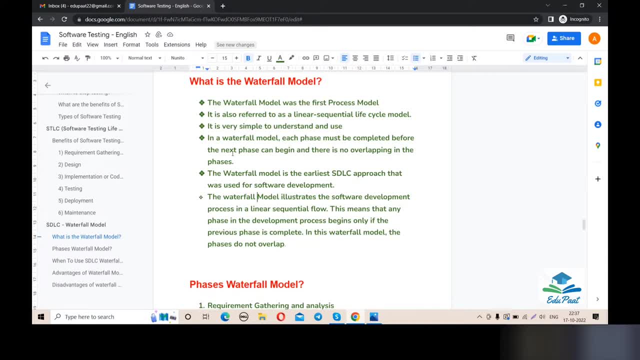 and there is no overlapping in the phases. okay. The next point is that the waterfall model is the earliest SDLC approach that was used for software development. As I have already told you, that waterfall model is the first process model. okay, So that means in the earliest SDLC approach is the waterfall model okay. 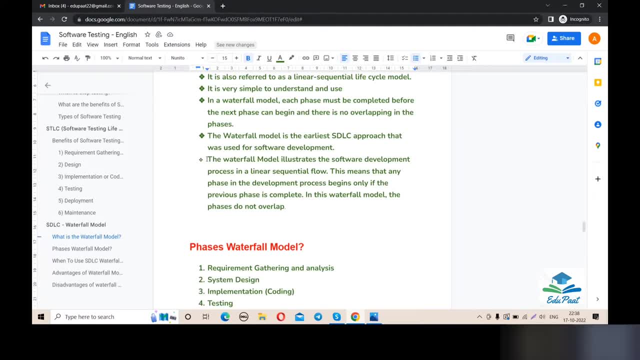 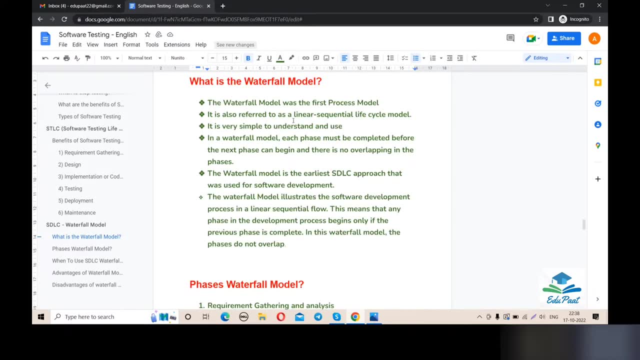 And the last point is that the waterfall model illustrates the software development process in a linear sequential flow. As you guys, I have already told you that the name of waterfall model is linear sequential life cycle model, right, So why the name is linear sequential life cycle model? 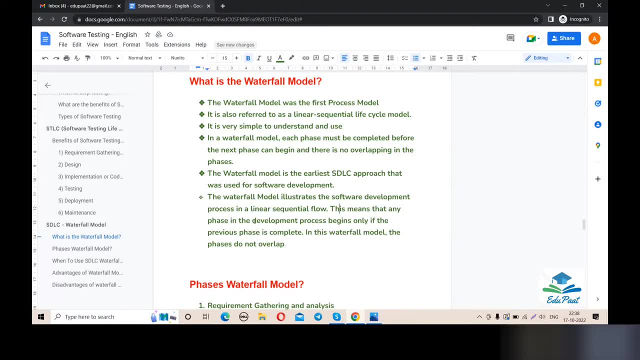 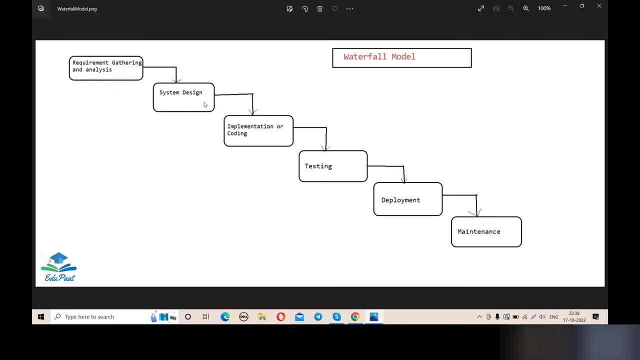 Because this means that any phases in the development process begins only in the first phase, Only if the previous phase is complete. So in this waterfall model the phase do not overlap. That means when one phase is running, then all the phases is not working. 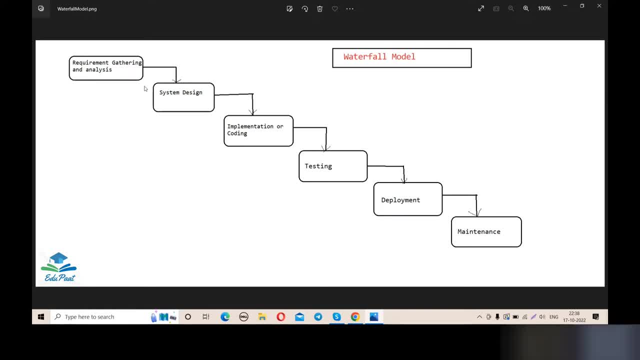 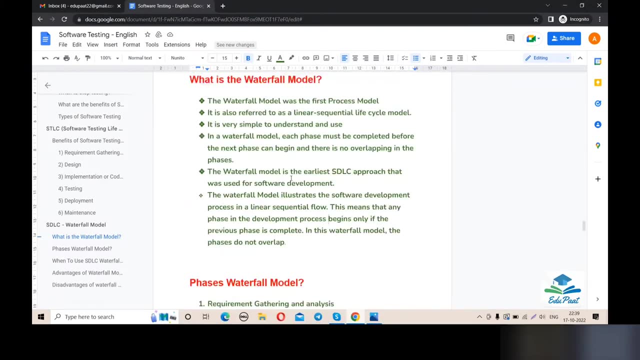 They will freeze or they will fixed When the requirement gathering and analysis phase will start, will begin. then the other phase will seated right. So that is the thing. So that is the thing on the waterfall model. So now you guys, now you guys can very clear about what is waterfall model. 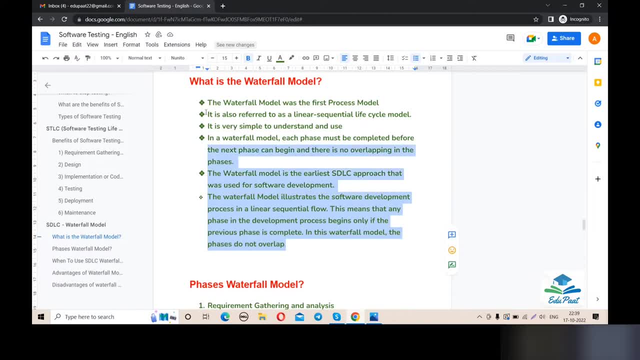 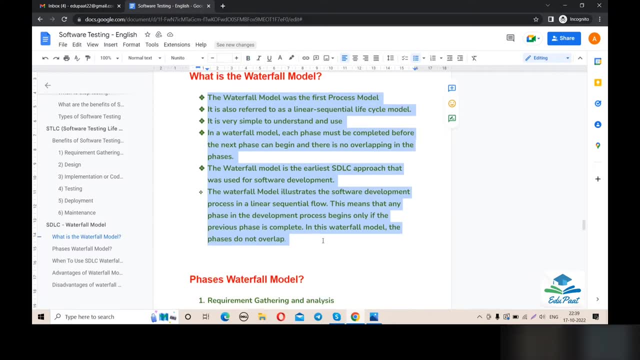 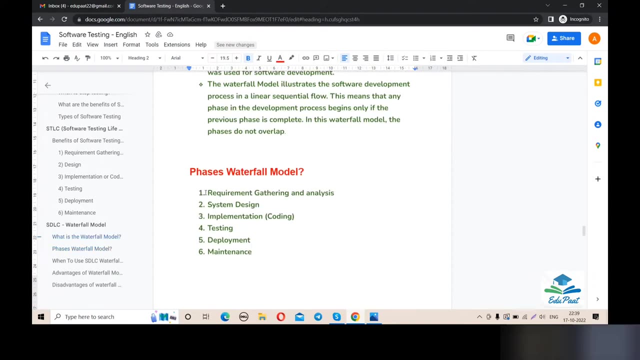 And for your helpful. I have already mentioned some few point So you guys can see all the point and you guys can remember. And the next next point is that what is the phases of waterfall model? Like there are six phases of that in waterfall model. 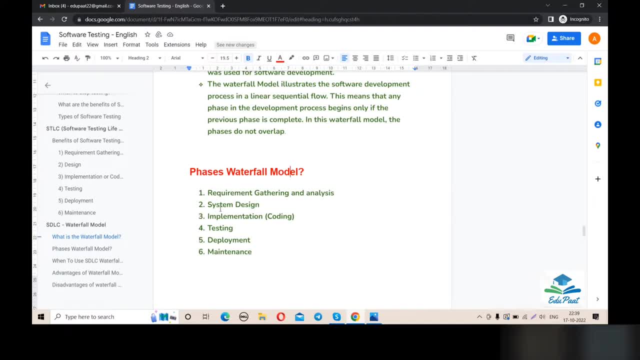 One is Requirement gathering and analysis. Second one is system design. Third one is implementation or coding. Fourth one is testing. Fifth one is deployment And sixth one is maintenance. So, as you guys see, as you guys see my last video in SDLC, 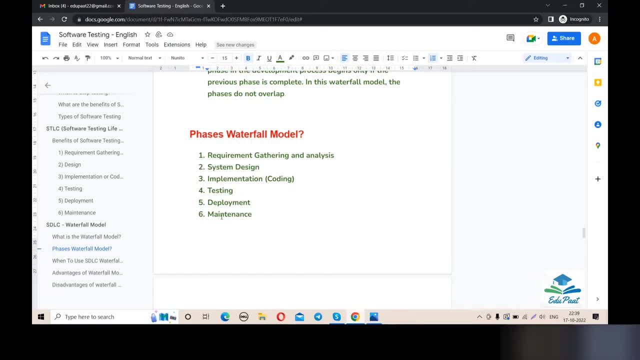 where I have clearly talked about the SDLC phases. Okay, So there is same like that. all the phases are same like. So you guys, if you guys already see my video, you can easily connect with both of these waterfall model phases and SDLC life cycle phases. 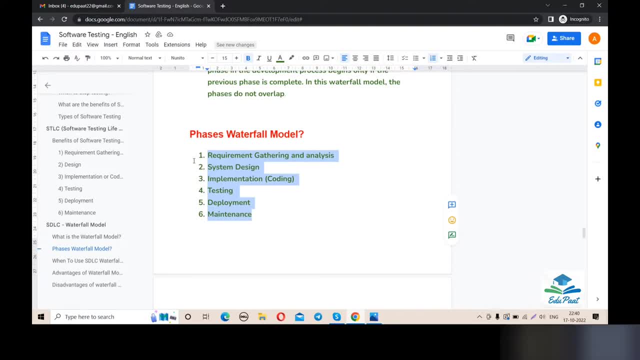 So if you guys not seen my videos till now, I'm requesting you that please see my the last video, SDLC video, or either I am giving the link in my description box So you guys can check from there also Now. So what is? 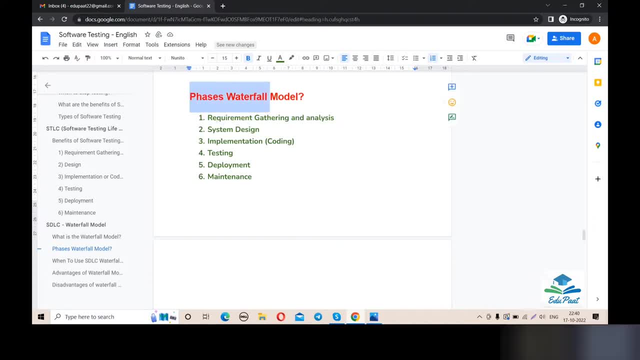 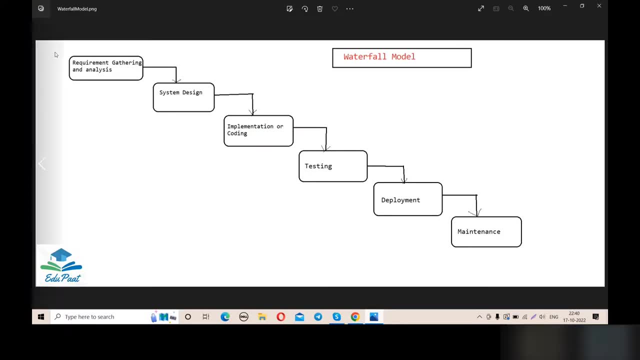 The requirement gathering and analysis, or phases of waterfall model. So I am giving, I am showing you one picture. So that is the flow in waterfall model. First one is requirement gathering and analysis. When it will be done, then the next phase will comes up. 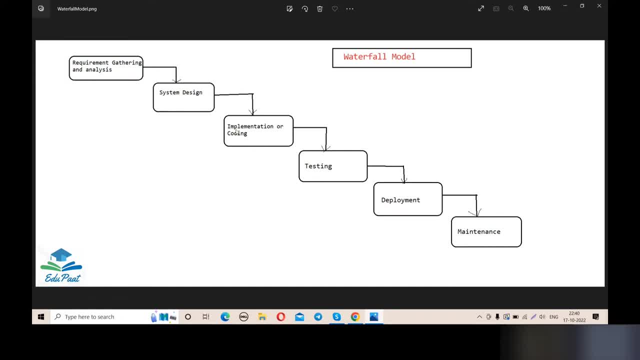 The name is system design. When it will be done, then the third phase is coming: Implementation or coding. Then fourth phase is testing, Then fifth phase is deployment And the sixth phase is maintenance. So that is the flow. So that is the flow. 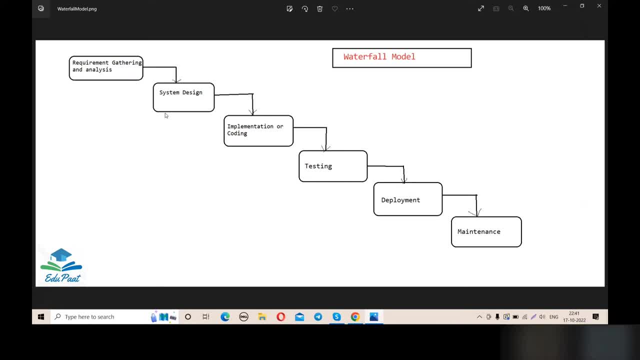 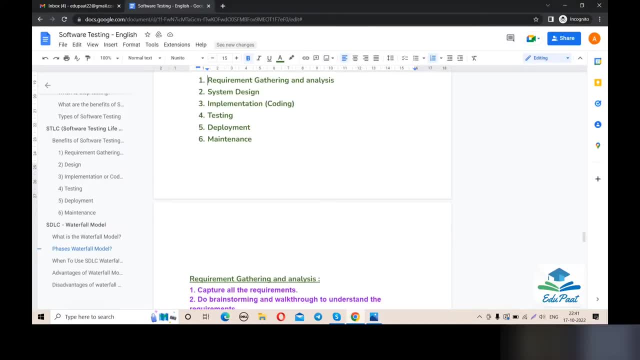 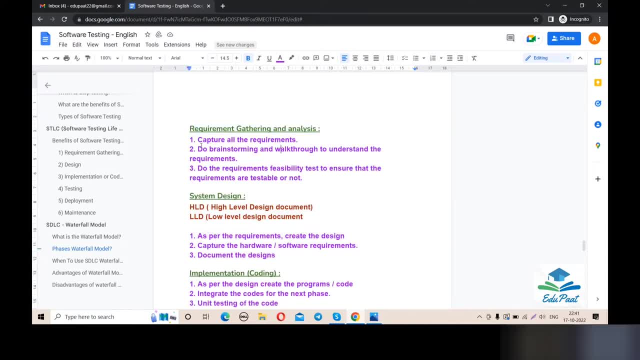 In the requirement gathering and analysis phase. capture all the requirements. Capture all the requirements. Do brainstorming and work through to understand the requirements. And the third is that: do the requirement feasibility test to ensure that the requirements are met. And the third is that: do the requirement feasibility test to ensure that the requirements are testable or not. 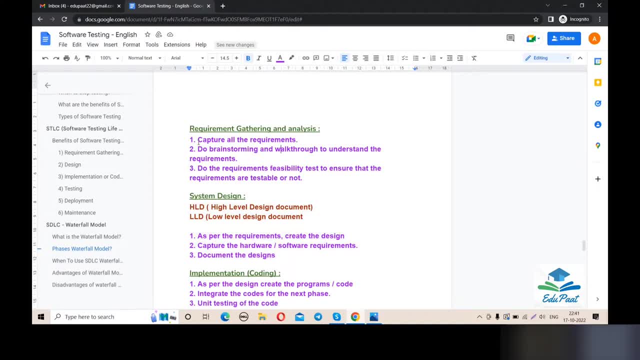 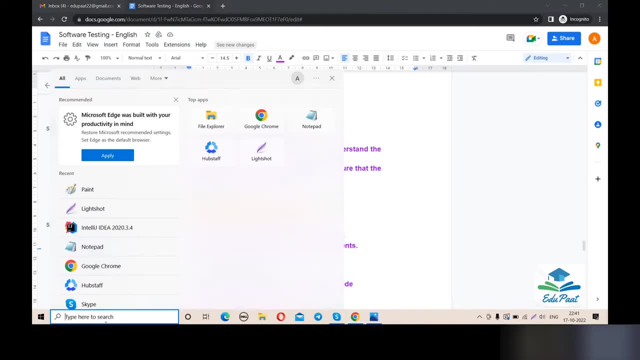 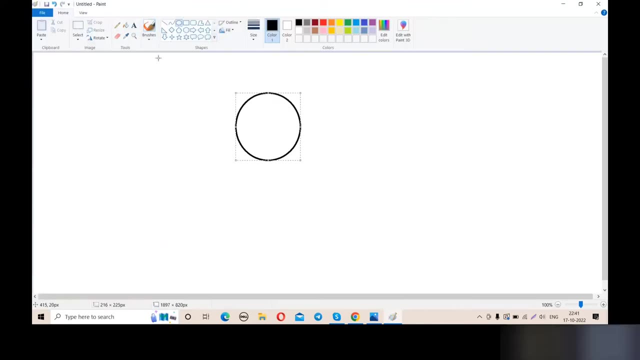 That means requirement gathering and analysis. So let's say: suppose there is a client or there is a customer. I'm giving you an example. Let's say: suppose this is my client or customer and this is a company. Let's say it's a customer. 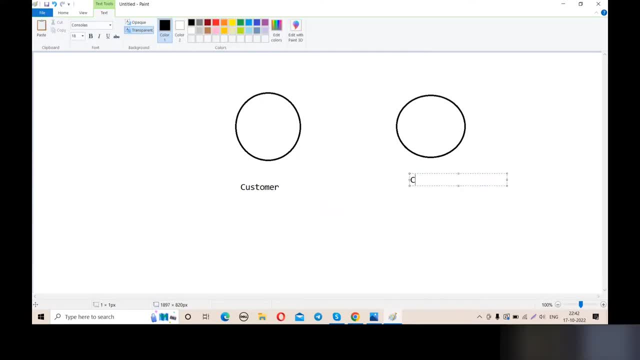 customer and this is the client. Company Now, company Now. thing is that what will be in the process of requirement gathering analysis Means the customer will give some requirement to the company, right. First of all, customer want to make some software or make some application. okay, That's why he contacted with some company. Let's say the company name is A and the customer name is B. okay, 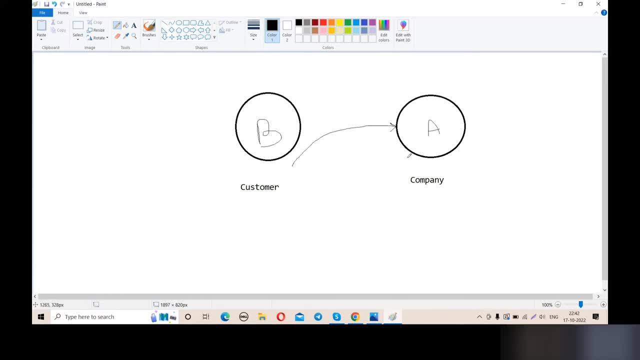 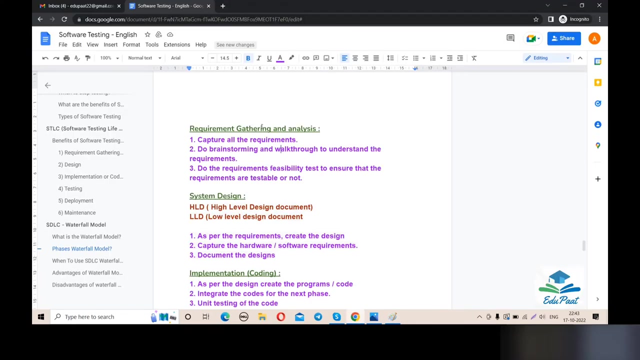 So then customer B will connect with the company A and he gives some requirement to the company. okay, Now that means in the company's BA or PA, means business analyst or product analyst, they will collect the requirement from the customer. okay, So in the phase of requirement gathering and analysis means the company will collect the requirement from the customer. okay. 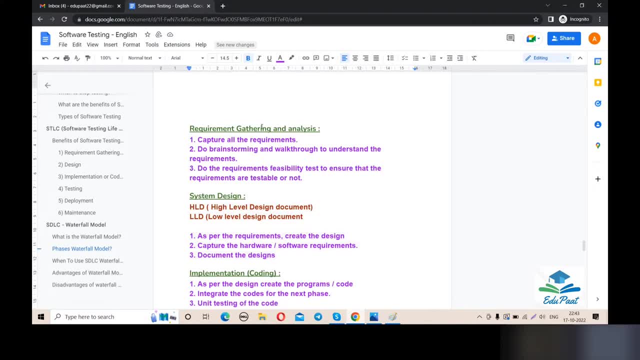 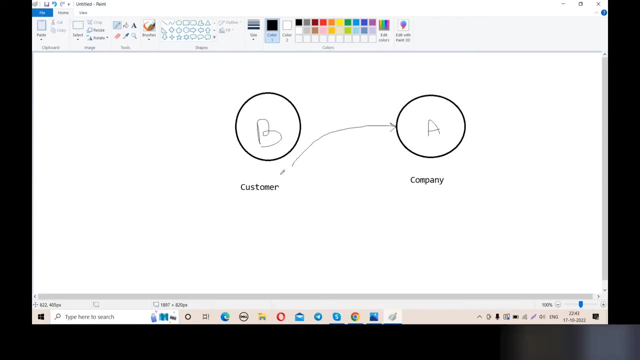 And they will do brainstorming and work through to understand the requirements right. And after that, what is the meaning of analysis Means? suppose the customer request customer says that the requirement already given, already given. then customer says that my time will be 30 days. let's say, 30 days in the 30 days you have to complete my requirement, or 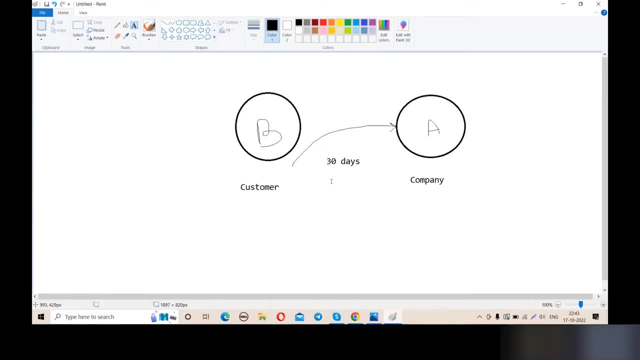 you have to complete my application and the budget will be, let's say, thousand dollar. let's say the budget will be two thousand dollar. okay, so then, and they told the company, like that, my, my, my applications language will be, let's say, php. suppose they have given some set of bundle? 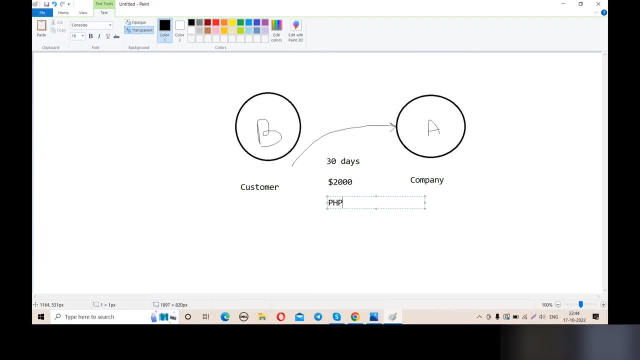 of requirement to the company. there are many more requirements are there, but as the example i'm just giving you some basic idea. okay, so then the customer, given this requirement, two thousand dollar, budget will be two thousand dollar. okay so then, and they told the company then what will do? first, companies ba or ph- they will collect the requirement from the customer. 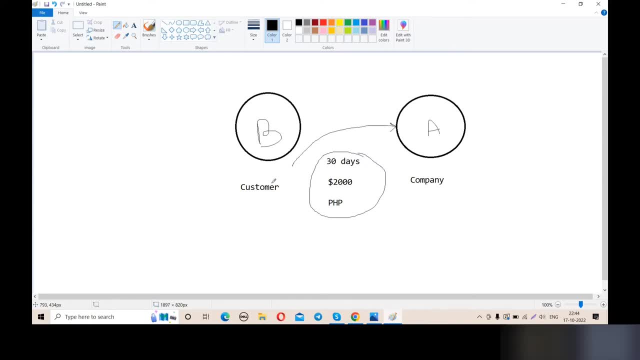 okay, then they will note down all the requirements and after that they will say that means after business analyst or or product analyst or the company's management. they will sit together in the internally. okay, they will sit internally. then they will give the requirement to the company and they will discuss all the things. that internally means the 30 days is possible to. 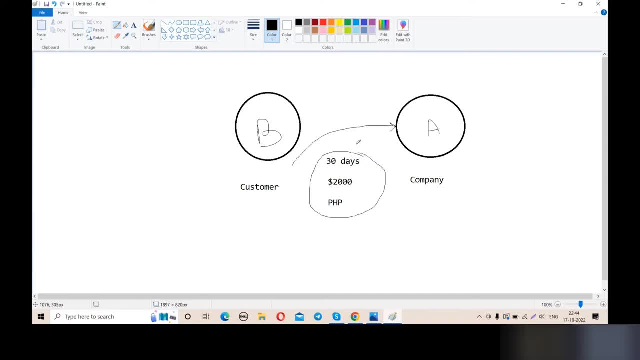 complete the software, or two thousand dollar is enough to complete the software or the language they have told. i mean customer told the language to php, so is that possible to do the php language or is there any resources are available, like many things are there, so they will. in the company we. 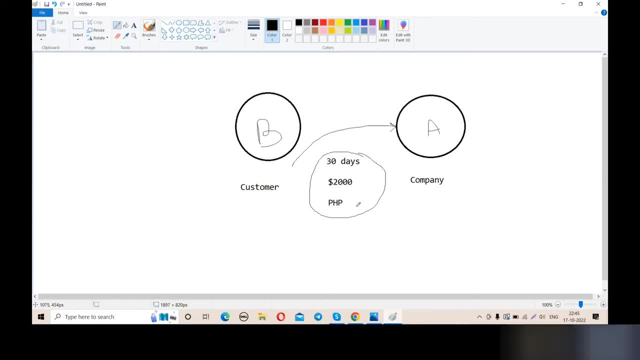 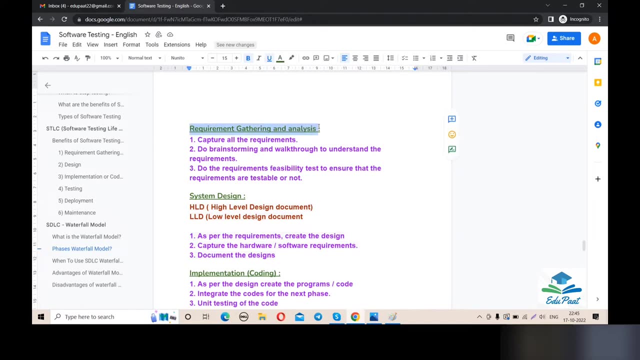 analysis, all the thing. that's why my first point is that they will discuss all the things that are requirement gathering and analysis. first they will capture our companies, ba or pa, will capture all the requirements, then do. then they do brainstorming and work through to understand the requirement. and the third point is that do the requirements feasibility test to understand. 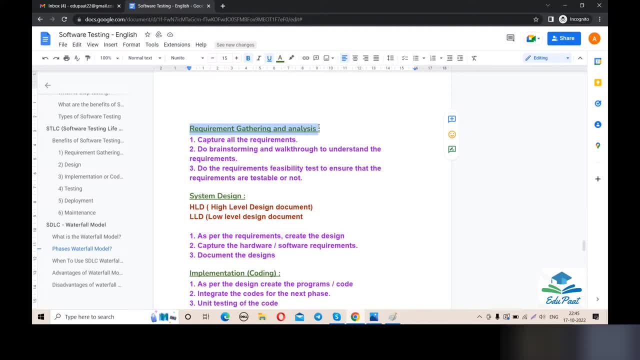 to ensure that the requirements are testable or not. many more things are there. okay, so that is the requirement gathering and analysis part. now what is the second point? the second point is that system design, system design means. system design means there are, there are two types of designers. 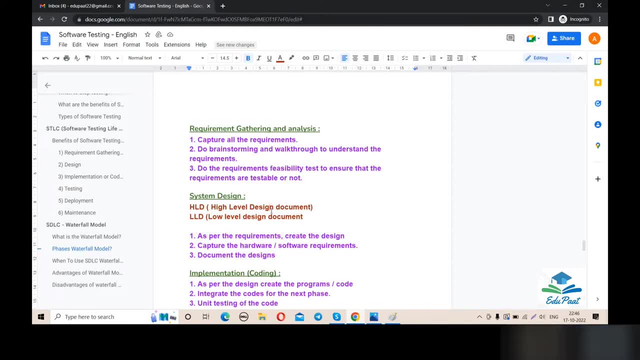 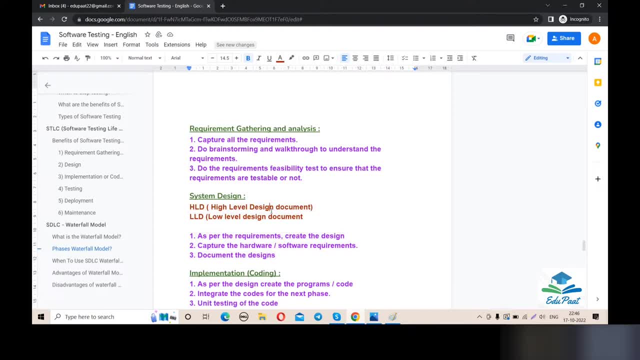 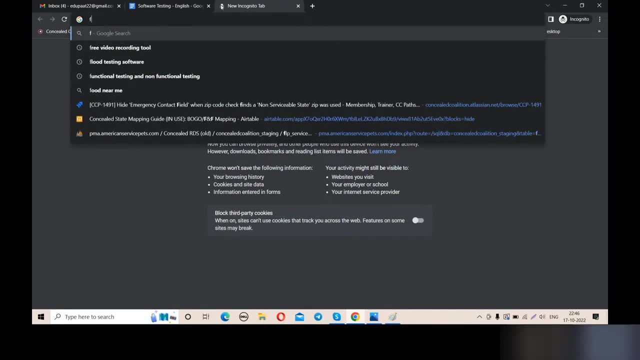 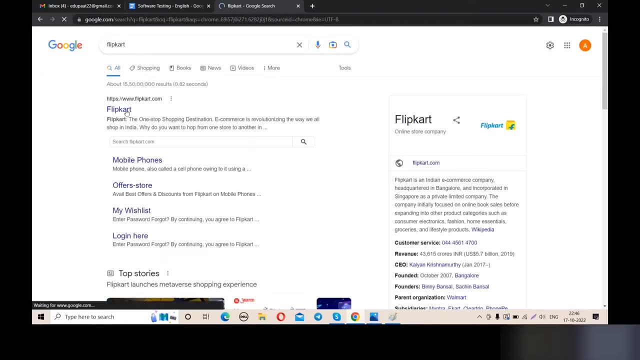 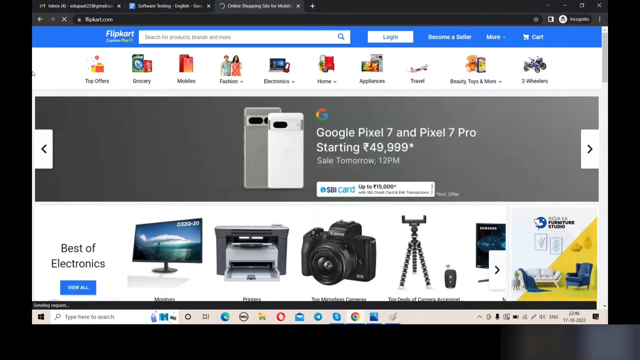 lld. guys, i'm giving you a very basic example. let's say: suppose i am opening one site called flipkart, let's say flipkart. what will happen? i am opening one site, flipkart. now what do you mean by hld? hld means as a user, i am, i am visible, what i am visible in my 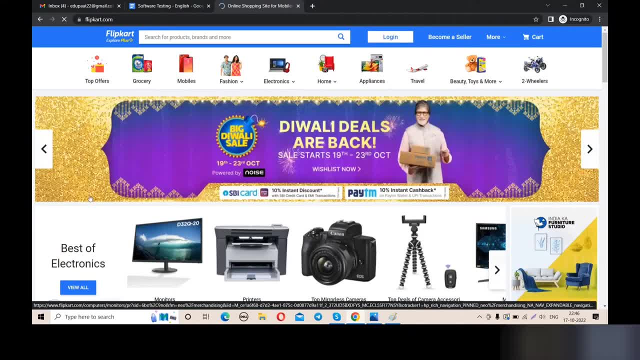 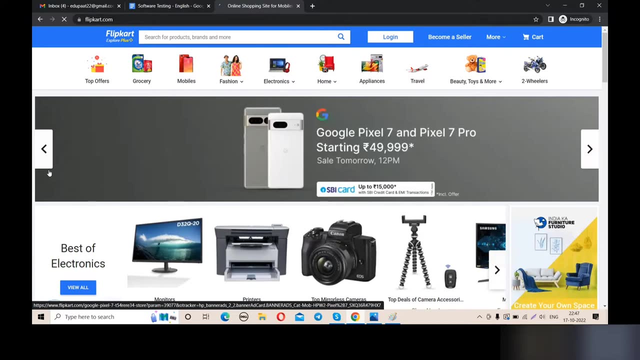 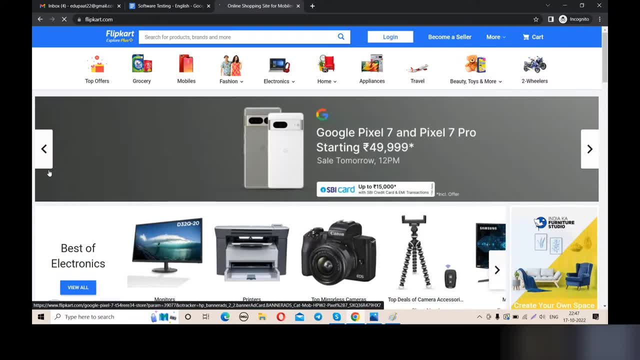 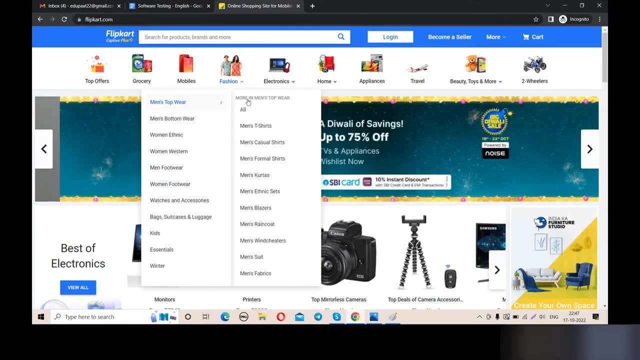 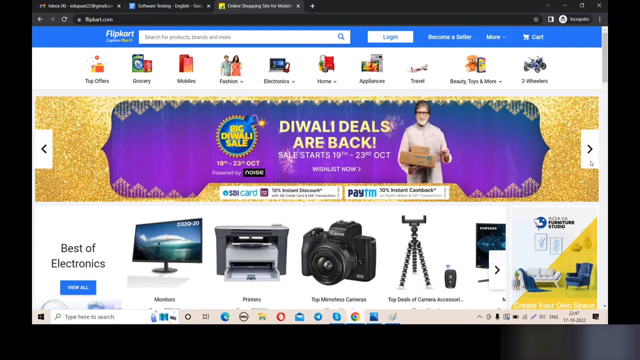 to us directly is nothing but a hld or high level. okay, and low level means suppose there is one drop down like that fashion. so so when i am hovering on this, when i am doing mouse over on the fashion, then few, few items showing up there. that means that is not visible in the first time when i am open the site or when 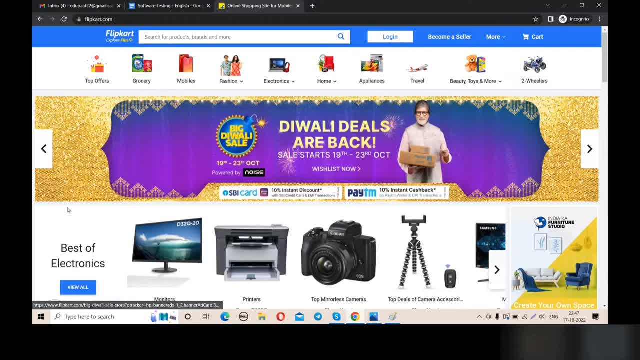 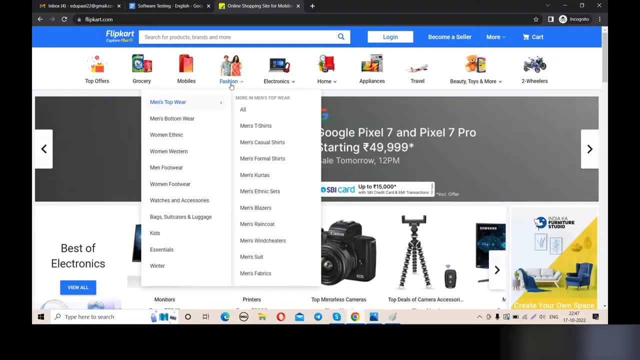 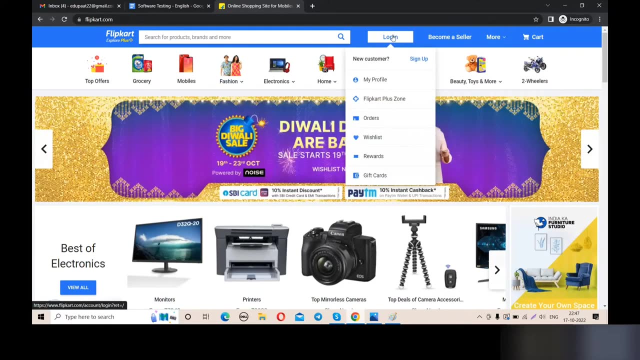 i am open the application, that is not visible to us. only this page is visible to me right, and when i am doing hovering anyone, there is few extra designers there, like when i am hovering on the more or anything. when i am clicking on the login, then one model is appearing. so that is all about. 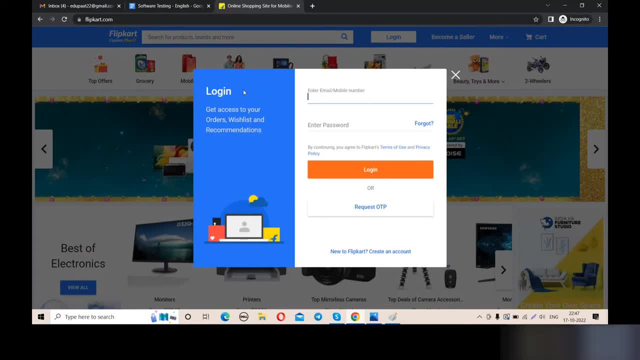 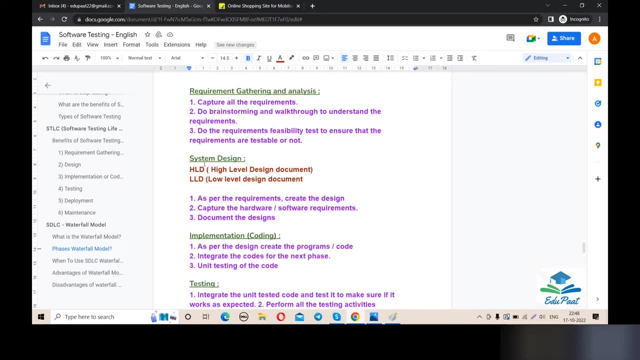 low level design. so now you guys can understand that what is high level design and what is low level design? so in the system design page there is two type of designing is there. one is hld and second one is lld. hld means high level design and lld means low level design. so what will happen? 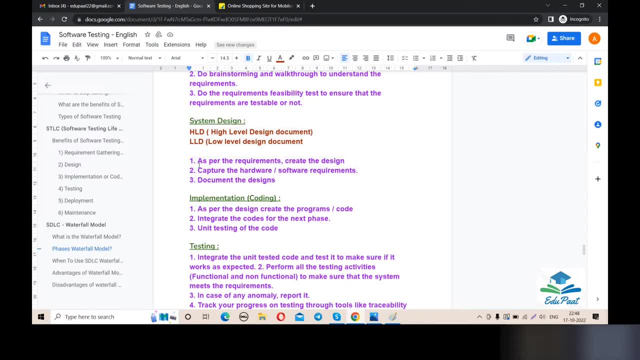 on the system design as per the customer requirements, create the design. what is the customer requirements? based on the customer requirement, the designing team or the architect, they will create some design then then capture the hardware or software requirement. so we have to capture the hardware and software requirements- what is the requirement for the hardware and software- and then document the 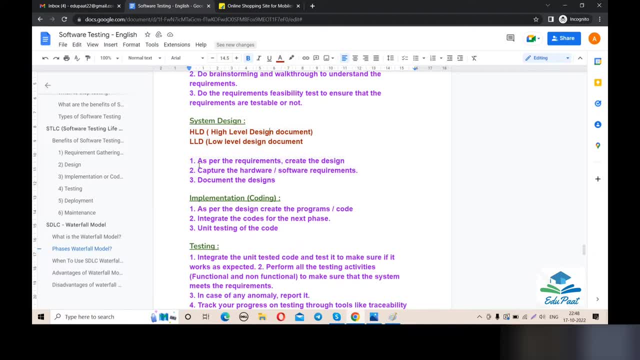 design, then we have to document the design, and then we have to document the design, then we have to document the design. our architect or designer, they will make the hld or and lld as per customer requirement. that is the system design page and the next point is that implementation or coding, 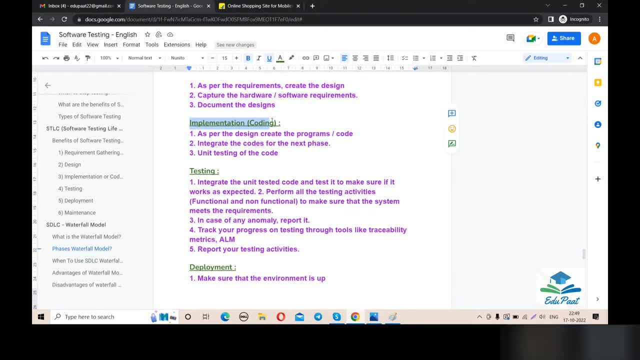 the naming says that we have to make some code. client has given some requirement to us, right? client has given some requirement to the company. then what will happen? designer will will make some design, makes some high level design or low level design. after get, after completing the design part, then the developer will. 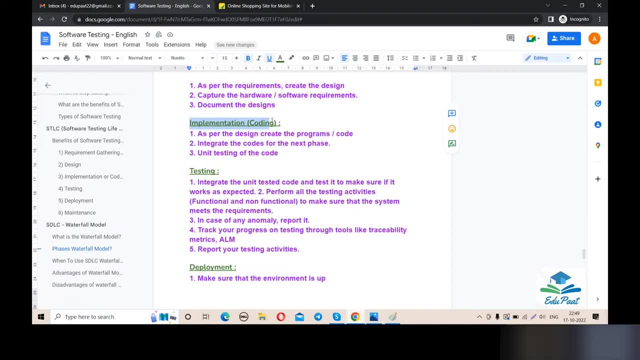 develop something they will develop to build or to make the software. so, in the implementation of coding phase, as per the design, create the programs or code right then. second point is that integrate the codes for the next phase. for the next phase, we have to integrate the code. 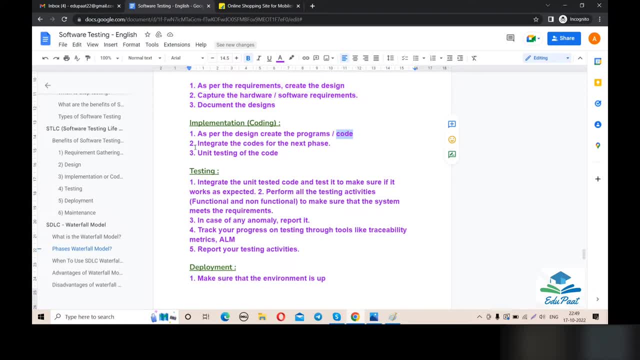 And the third point is unit test of the code. Why the unit testing of the code? So in my next video I talked about in details what about unit testing. But as of now unit testing means that developer- suppose developer- writes some. 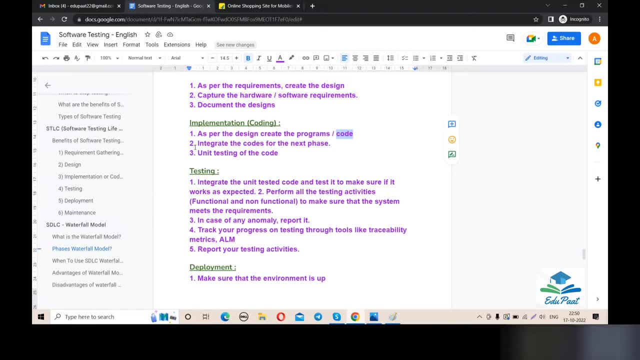 written some code and the code is working perfectly fine or not. who will check? The developer will check. So when developer will check? or when developer will test something that is called unit testing, Right? So in the implementation or coding phase, as per the design. 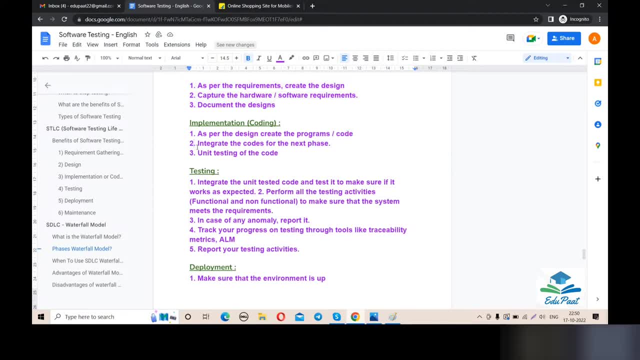 create the programs or code, then integrate the codes for the next phase and then unit testing of the code. Okay, Now clear. The next point is that the next phase is that testing. Testing means after completing the coding, after completing the unit test by the developer. 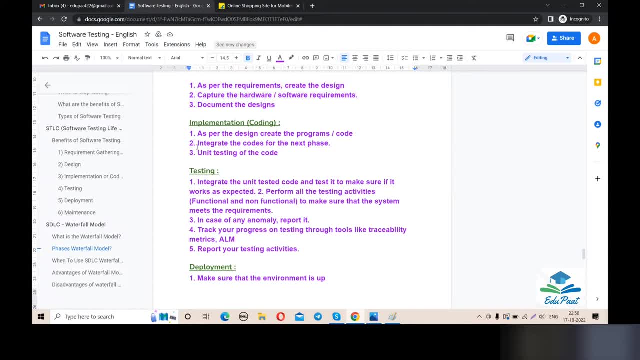 then they will hand over the software or application to the test Testing team. Then what will do Testing team? will test the application thoroughly. They will do various kinds of testing like regression testing, smoke testing, sanity testing, integration testing, performance testing. 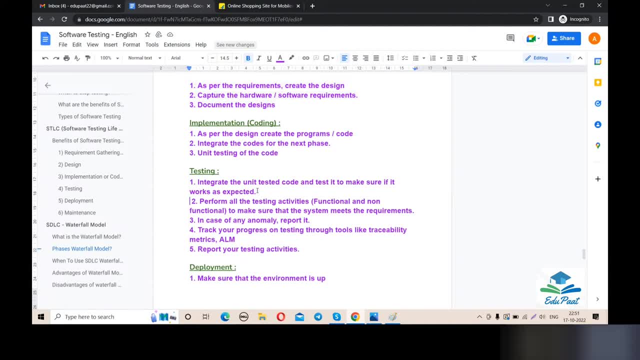 means functional testing and non-functional testing. So in my next, in my later video, I will tell you all the things in very easy way, So don't worry about that. In the testing I am just telling you that what we will do in the testing phase. 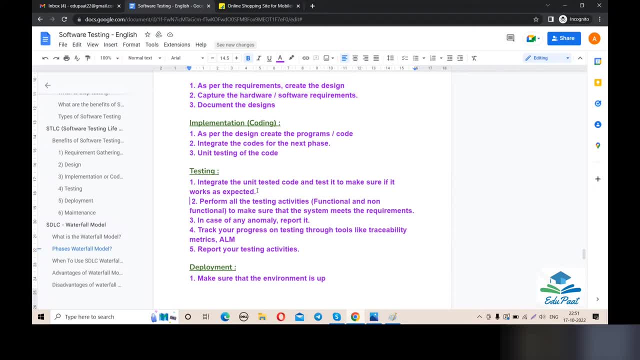 First point is that integrate that unit tested code and test it to make sure if it is working as expected or not. That means when we are testing something, when the testing engineer or when the testing team will test something that will be matched with the customer requirements. 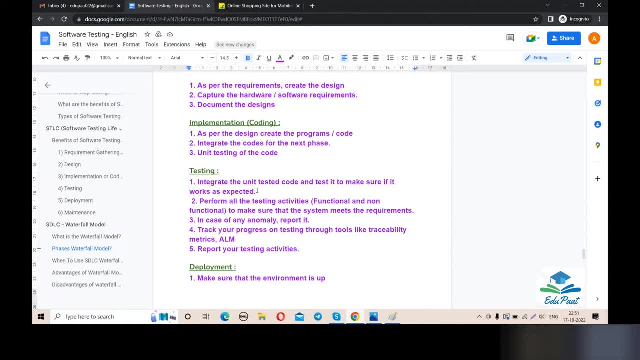 In my previous video. I already told you guys, the developer will develop the application as per the client's requirement or customer requirement. The same thing is for the testing team. The testing team will test the requirement as per the customer requirement. That is the first criteria. 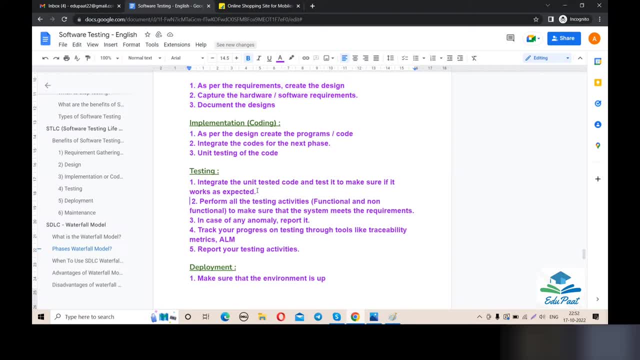 After customer requirement, the testing team will do various kinds of testing, like functional testing, non-functional testing, the non-functional testing, performance testing, security testing, many testing they can do, But first point is that my client's requirement or my customer requirements. 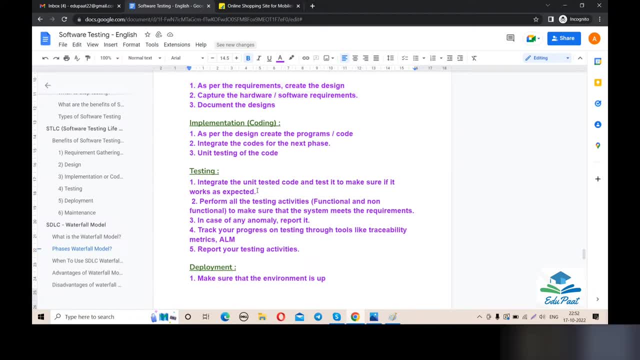 is working perfectly fine or not. That is the first thing. That's why integrate the unit tested code and test it to make sure if it is working as expected or not. Now second point is that perform all the testing activity. I have already told you that: functional testing, non-functional testing, 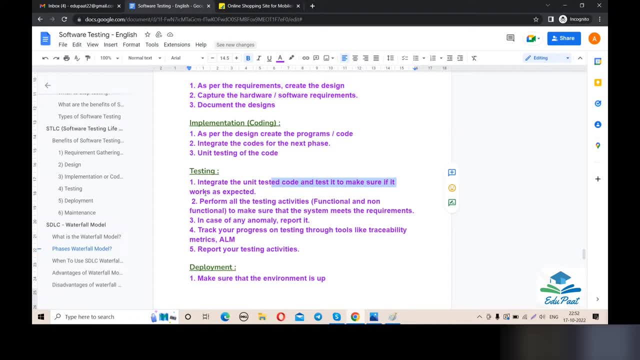 Perform all the testing activity to make sure that the system meets the requirement. The third point is that in case of any anomaly reported when we are testing something, when we are testing the application, if there is any bug or any defect, then first we have to report that. 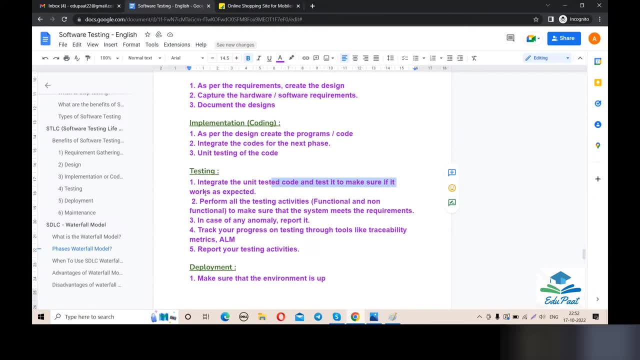 Then the developer can fix that code and again we can testing that. Fourth point is that track your progress on testing through likes to likes, testability matrix or ALM. So testability matrix or ALM is the tracking process tool where we can track our progress on the total testing right. 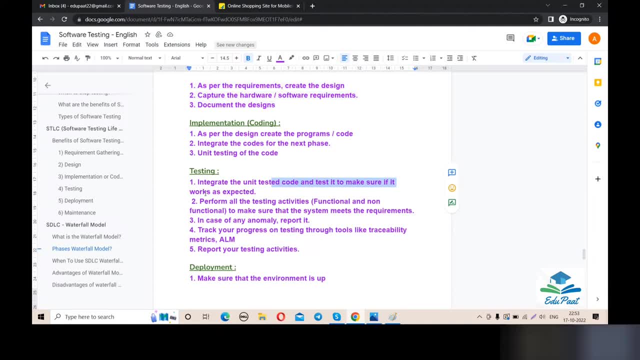 Then, number five: report your testing activity. We have to report our testing activity to whom? To my QA manager, or testing manager, or my team lead, right So? or my client or my customer. I have to report my testing activity, that how many test case I have passed and how many test case I have failed. 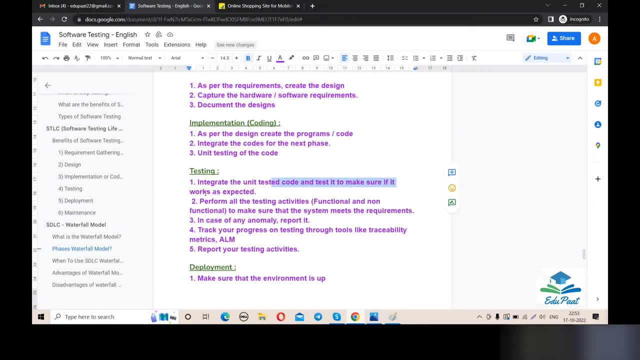 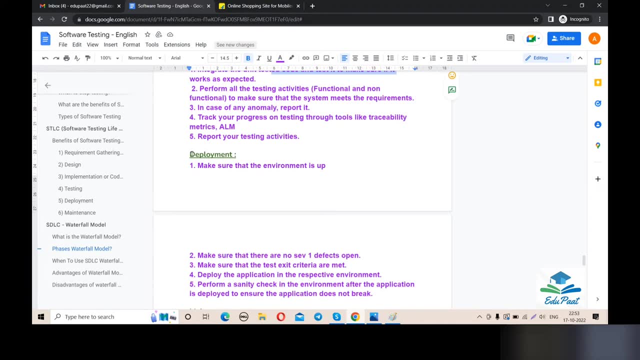 Right. So that is the testing phase of waterfall model. The next phase is that deployment. What will be done in deployment? First point: make sure that the environment is up. Deployment means when the testing is passed, Means the test engineer tests all the criteria. 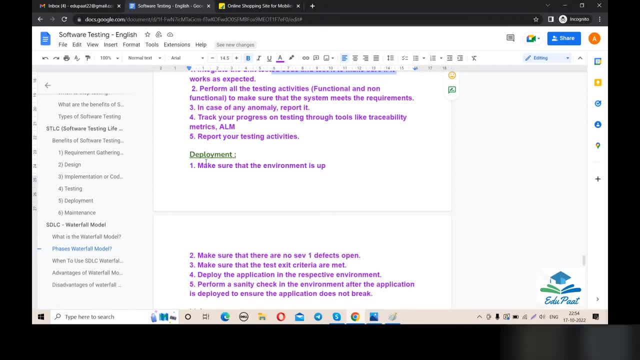 they have matches, all the clients requirements and if they get signal, If the testing team, testing team team sign out, him sign up the application, mean all are working. all are working, perfectly fine. then obviously we have to deploy the application to ut environment or production environment, as 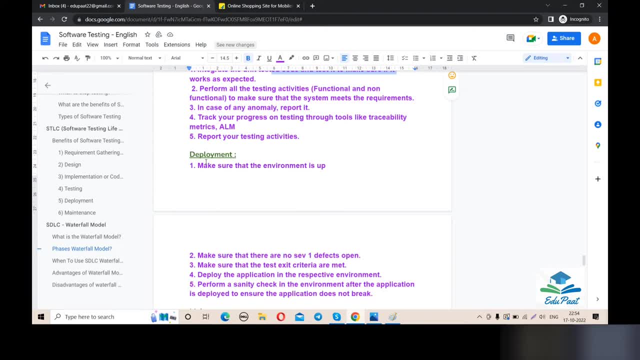 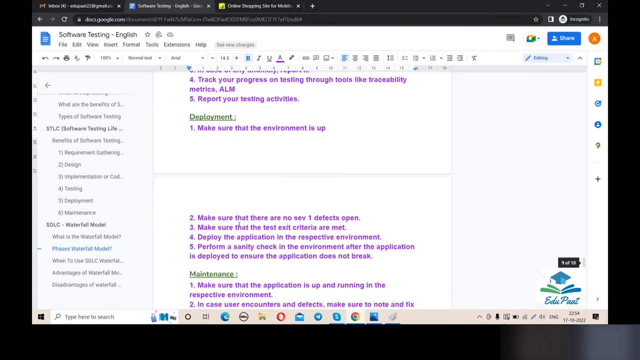 for the client or customer requirement or customer request. so we have to deploy that. so first point is that make sure that the environment is up. the second point is that make sure that there is no save one defects. open means we have to make sure that there is. 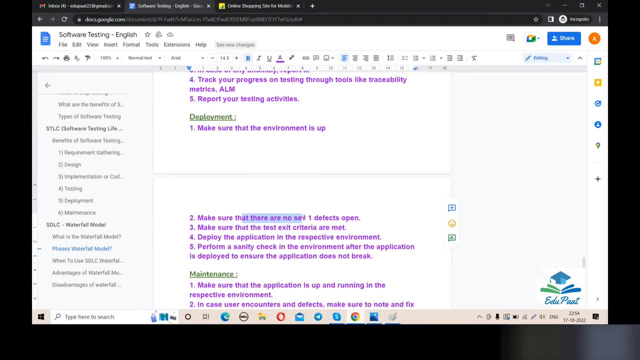 no severity defects. open means. severity means the the impact of business. if there any bug that is impacting my business scenario, that is called severity. so in my later video i talked about in severity, in severity in very details, but as of now, severity means the you Hyun생. 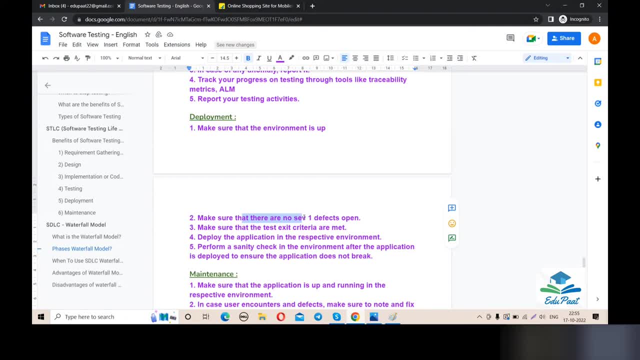 awakens impacting of the business scenario, if there is any. if there is any bug that is impacting my business scenario, if that is, then defects should be open. make sure that there is no severity defects open. right third point is that make sure that the test exit criteria. 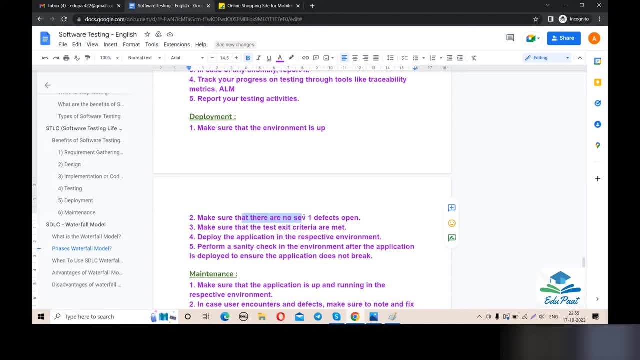 are met. so what is the test exit criteria we have to make? right forth point is that deploy the application in the respective environment. as for the client or customer requirement, for the client requirement, if the client wants that- you uh that we have to deploy the application to the uat environment, then obviously we have to. we have to deploy the that application to the uat. 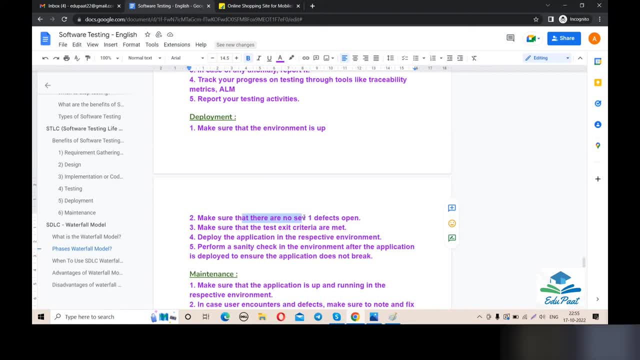 or if they, if they request to deploy the application to the production environment or live environment, then we will deploy the application to the live or production environment. so that means deploy the application in the respective environment. and then, last point, is that perform a sanity checking, sanity testing in the environment after the application is deployed, to ensure the 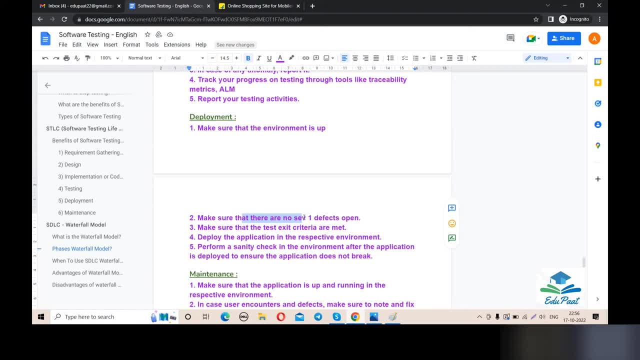 application doesn't break. so what is sanity testing? i will talk to you later, but as of now, after deploying my after deployment, then we have to test the application in a very basic way: that the application doesn't break, we have to check some critical functionality. okay, that our application doesn't break, we have to check that. 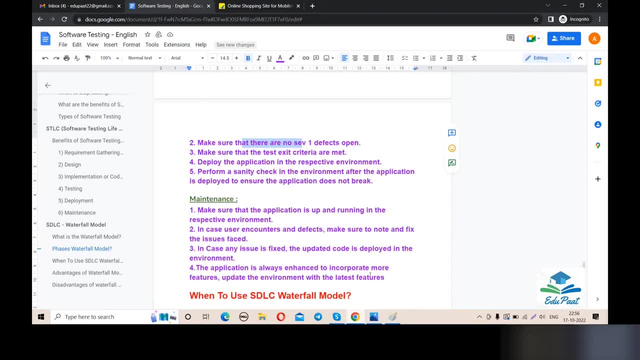 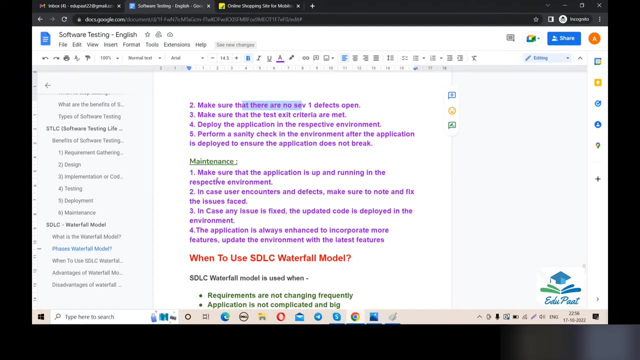 okay, and the last phase is that: maintenance. so this is the last phase: deployment we have done, then we have the last phase- is the maintenance. what we'll learn in maintenance page- make sure that the application is up and running in the respective environment- means application we have deployed. we have deployed the application as far there as 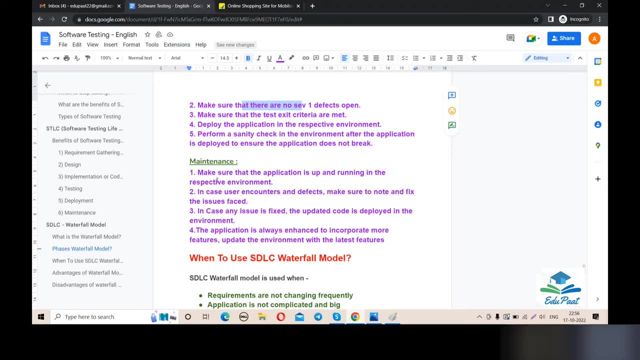 for the client respective environment or a client request respective environment. we have already deployed that and in the maintenance we have to make sure that in that environment- respective environment- the application is up and running. the second point is that in case of user encounters and defects, make sure to note and fix the issue first, if any. 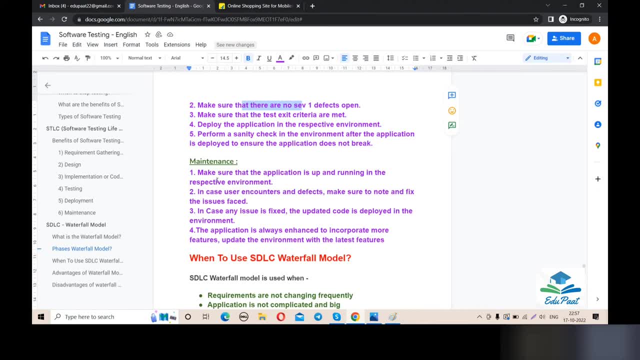 user is facing any type of issues or if any user they are getting any bug, obviously we have to note that bug and as as a pirate you have to fix that bug, so that bug should be fixed first. right and number three in case of any issue is fixed. 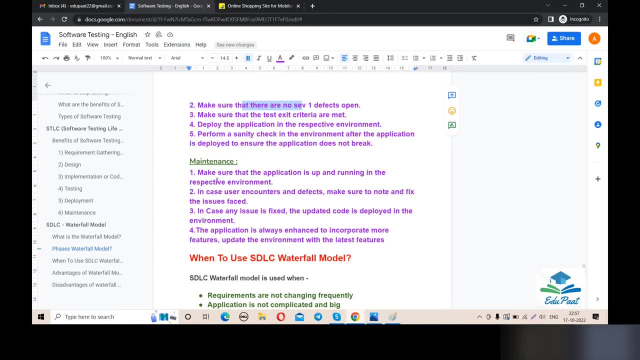 the updated code is deployed in the environment means if the, if any user getting any type of issue, then obviously they will report to our team. now, our team will fix that, the company will. the company's team will fix that. then, after fixation, we have to make sure that we have tested the. we have tested the. 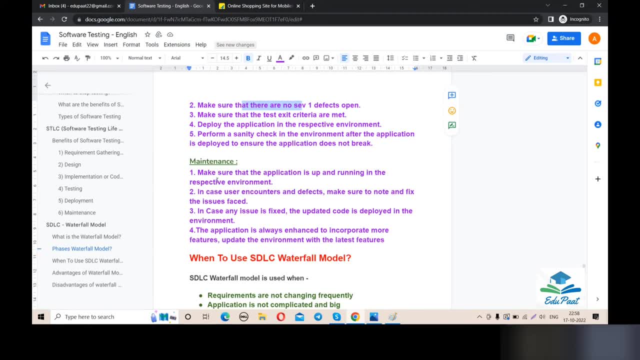 issue and after testing is first, then again we have to deploy that in the respective environment. and the last point is that the application is always enhanced to incorporate more features, update the environment with the latest feature features, obviously for the tacking purpose. we have to make some version so that we can track or we can update the environment with the latest. 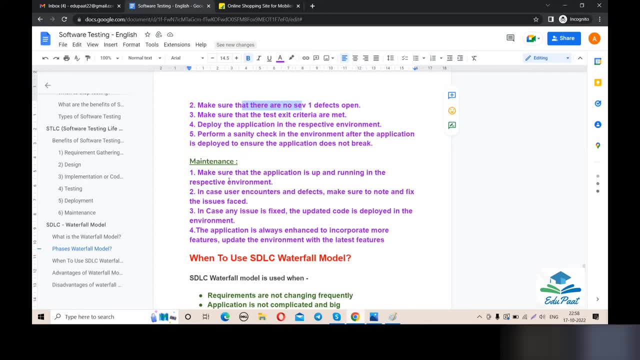 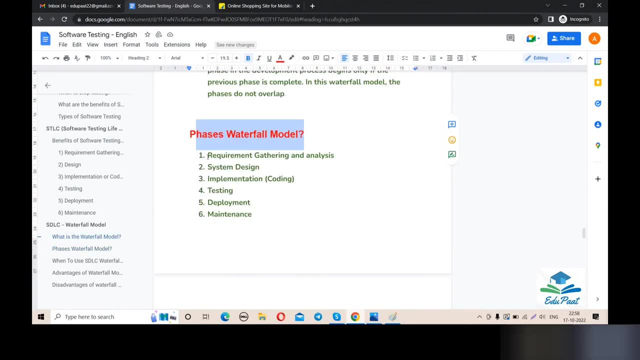 feature, right. so that is the. that is the thing of uh, phases of waterfall model. so now you guys is very clear about what is the waterfall model, what are the phases of waterfall model and exactly what activity will be done in the different phases of waterfall model. now next point, next topic, is that when to use sdlc waterfall model, when we 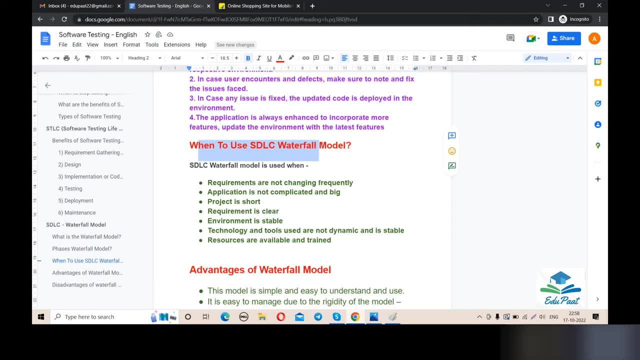 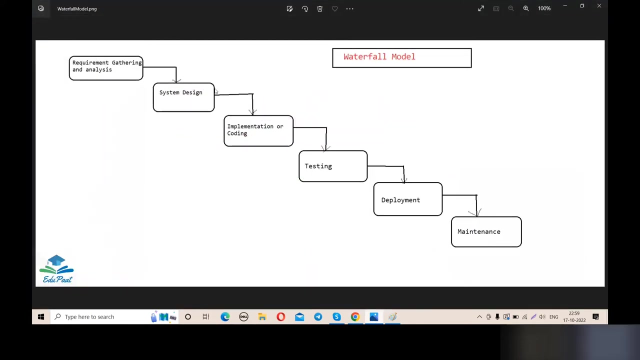 when we will use or when our company will use the sdlc waterfall model, when first, when the requirements are not changing frequently means, as i have already told you, that in the in the waterfall model, when one phase will done, then the next phase will start. then like that. so when one phase will done, we cannot revert back to the. 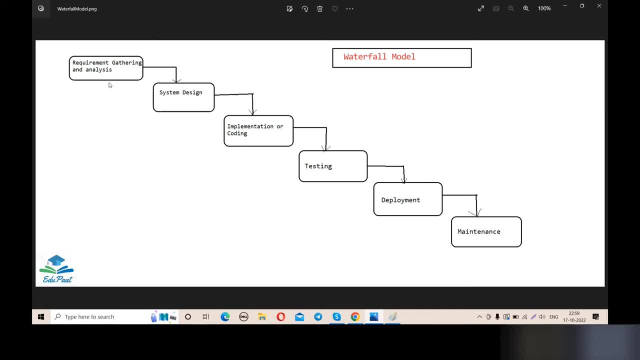 previous phase. oh sorry, we cannot revert back to the previous stage. that means when the requirement gathering and analysis part is done and system design part is started, that means we cannot revert back to the requirement gathering or analysis phase. so if there is any issue is happening on that phase, on the previous phase, 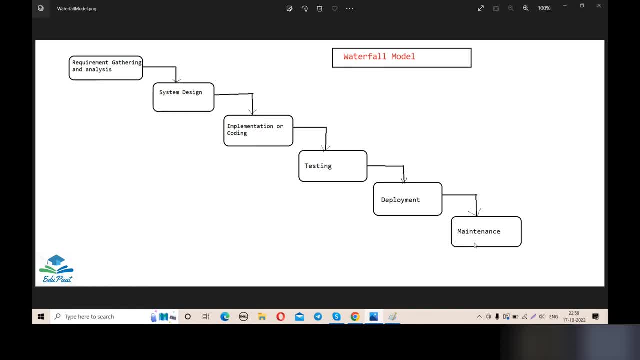 all the things will be solved in the maintenance phase only. that is the funda of the waterfall model. so when one phase is done and the next stage will be start, so we cannot revert back to the previous stage, or if we getting any issues, then obviously that will fixed on the maintenance stage. so when 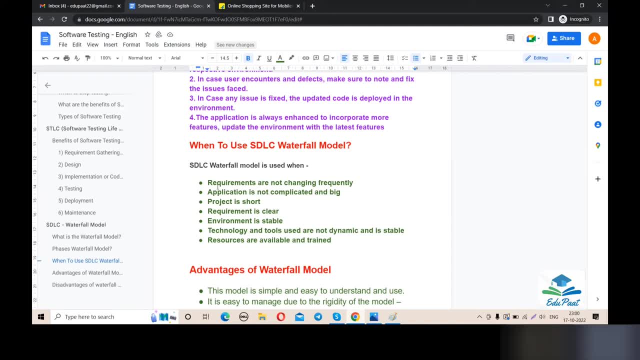 we use the waterfall model when the requirements are not changing frequently. application is not complicated and big. for the for the small application, we will use the waterfall model. application is not completed, not complicated and big. the project is short, requirement is clear, environment is stable, technology and tools which are which were used are not dynamic and stable. 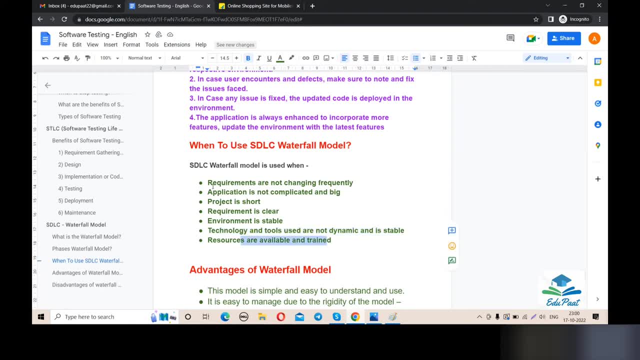 or resources are available and trained, that time will not use the sdlc waterfall model. so that is the theme of, that is the fund of sdlc waterfall model. so when we will use sdlc waterfall model, that is the main thing. when the project is short, when the requirements are clear, when the environment is stable, when the technology 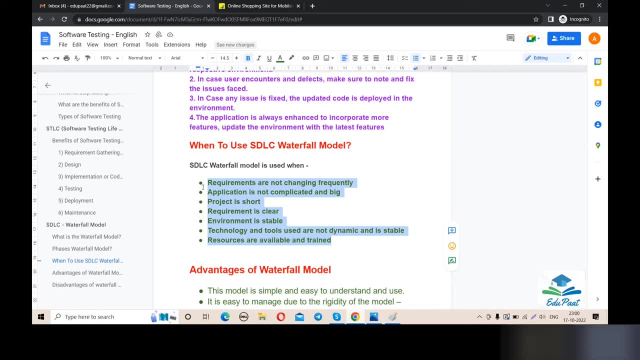 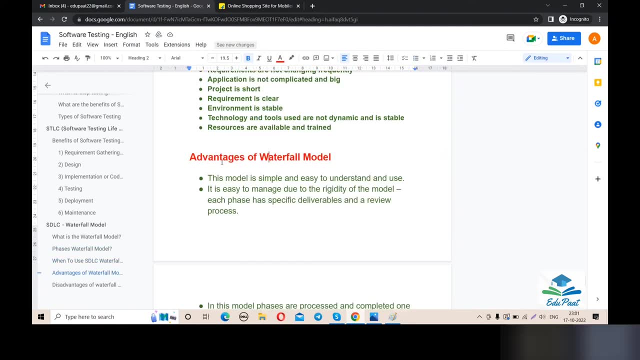 or tools are used in dynamic and stable or when the resources available are attained. so then we will use the sdlc waterfall model. then advantages of waterfall model. so what is the advantage? the model is simple and easy to understand, as the picture says that it's a very 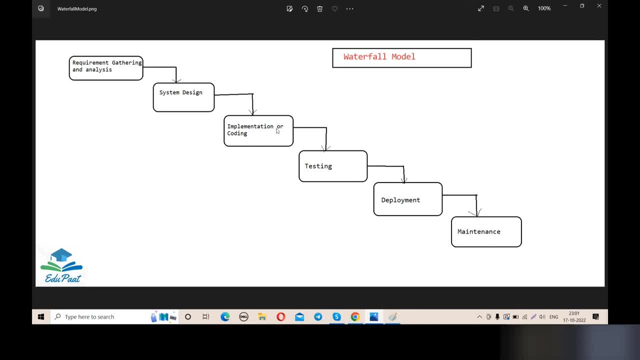 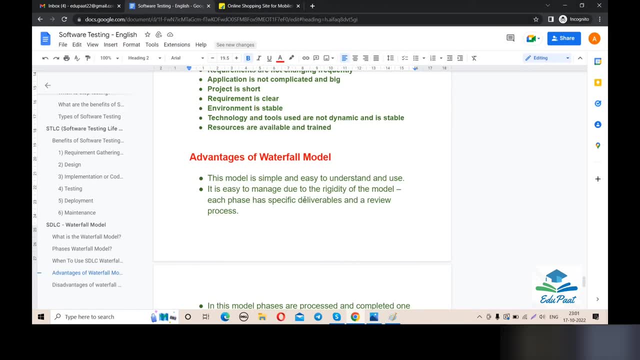 easy model. first we'll collect the requirement, then design, then coding, then testing, then deploy the maintenance. so very easy, very easy way and very easy model. so it's a very the model is simple and very easy to understand or easy to use right. second point is that it is easy to manage due to rigidity of model. 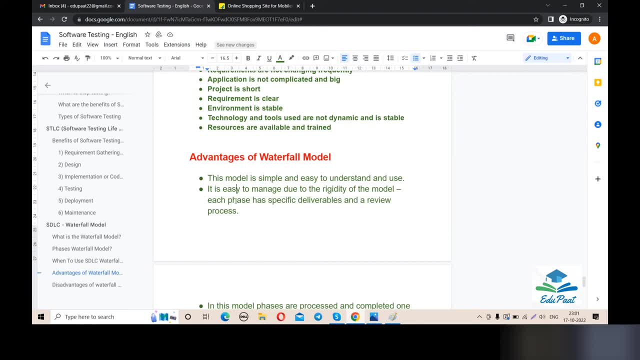 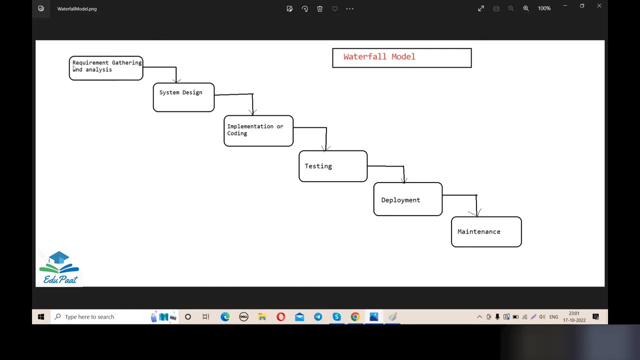 means each phase has specific deliverables and a review process. that's why it's a rigid model, means why each phase has specific deliverables and a review process, because when requirement gathering is, an analysis is happening, then system design will not happen. that means after one phase is completed, then the next phase. 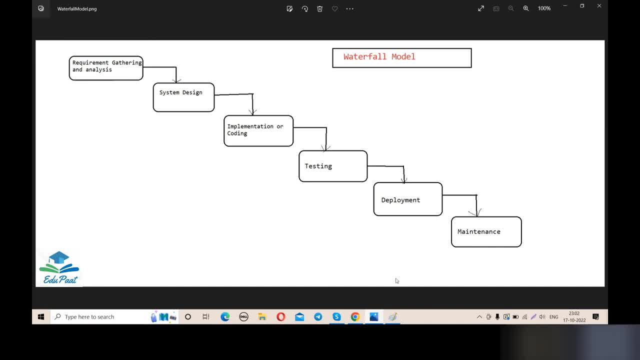 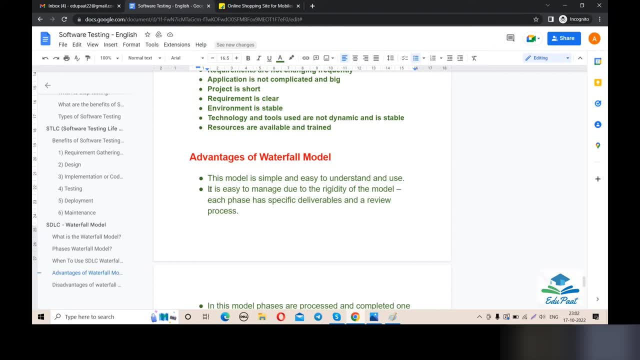 will start. that means it's a rigid model, right? so that's why i'm telling you that it's a easy to manage due to the rigidity of mode model. okay, and the third point is that, in the process of manage due to rigidity of model, 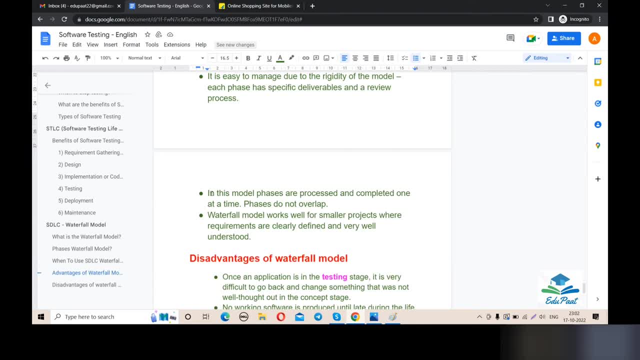 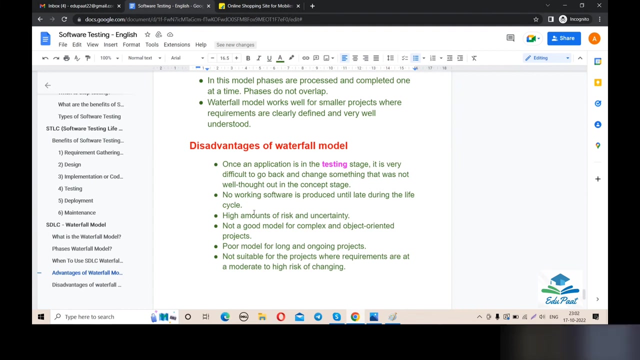 that in this model, phases are processed and completed one at a time. phases do not overlap, as as already guys, i have already told you that why the phases is not overlapping. third point is that waterfall model works well for smaller project where requirements are clearly defined and very well understood. right then? disadvantage of waterfall model? many disadvantages are there. 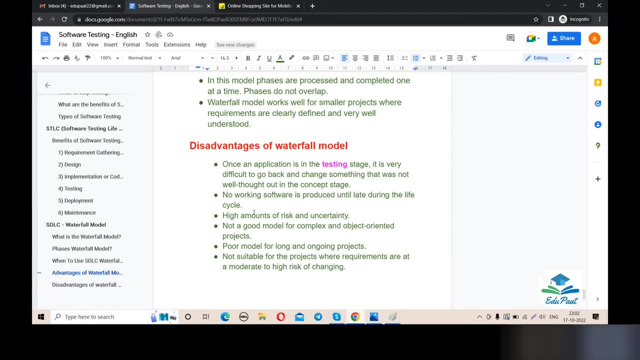 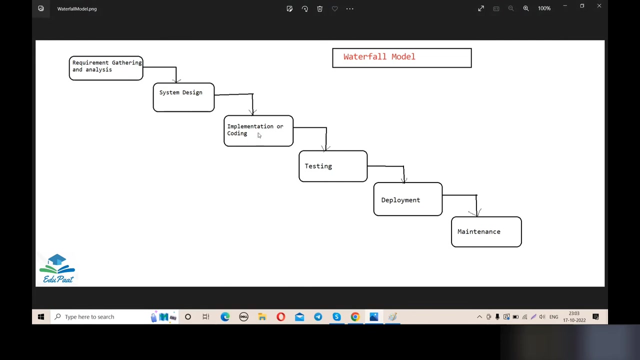 once an application is in the testing stage, it is very difficult to go back and change something that was not well through out in the con, in the conceptage. that means- suppose i have already told you that why? because when, suppose? i am on the coding phase so we cannot revert back to the design phase. so when our developer will? 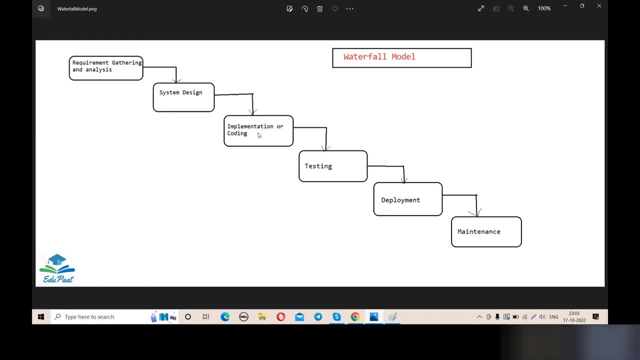 will do some coding. when the developer, they will start the coding. if there is any issue on the design phase they doubt, the developed team cannot revert back to the designing team. so that is the very disadvantage, right. so that's why, once the application is in the testing phase, 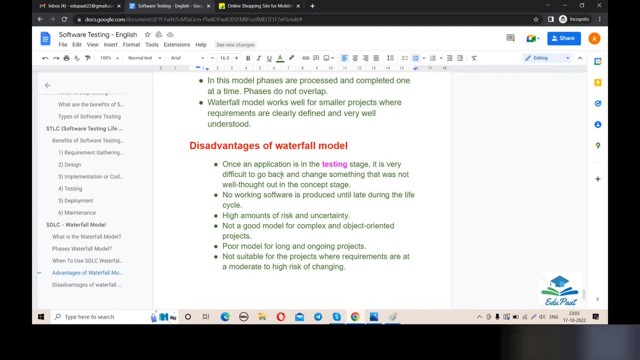 it is very difficult to go back and change something that was not well through, well thought out, on the concept stage. the second point is that no working software is produced until late during of the life cycle. right third point is that high amounts of breaks and uncertainty. why the high amounts of leaks? 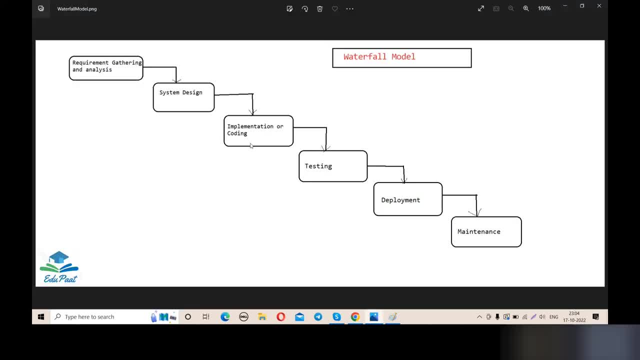 suppose i've. as i have already told you, one phase is done, the second phase will start and we cannot refer back to the previous phase. so if we can do that, that's exactly correct. so that means if there is any issue on the previous page, that will be not solved. that will be solved only on 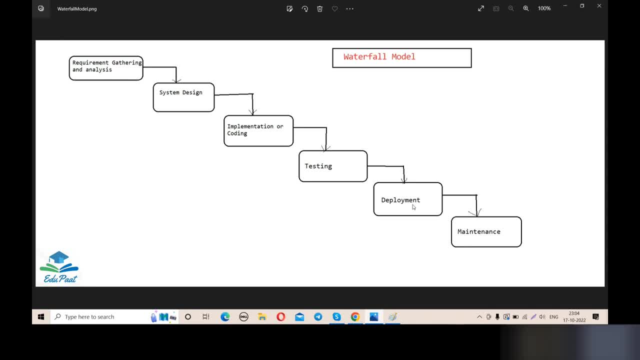 the maintenance phase. that means after deployment. so it was very risky. so as i already deploy my software to that live or to the uh, to the worldwide, so if there is any issue, all user can see that, see that, see that issue. so that is the uh. i mean not a good practice or that is the not. 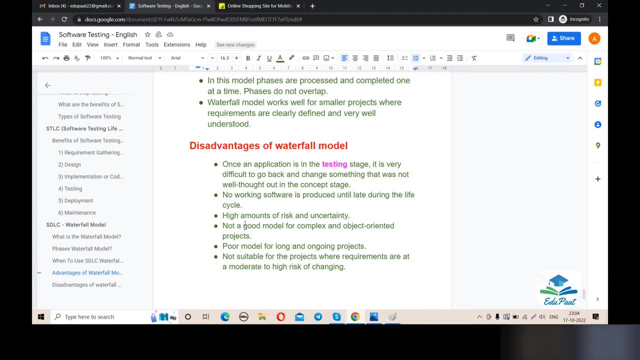 a good way. so that's why it's the, it's the high amounts of bricks and uncertainty. the next point is that not a good model for complex and object oriented project. if there is any complex project, so that is not a good model, then we have to think about some different model. and what is that model? 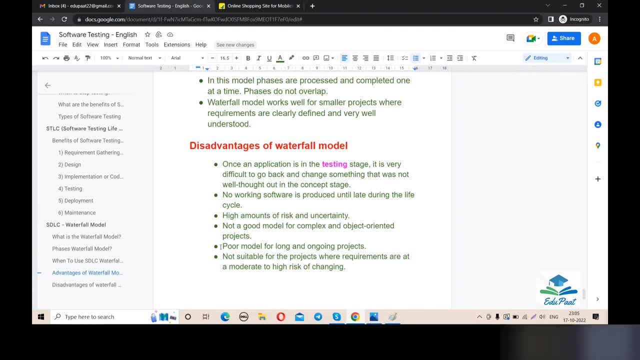 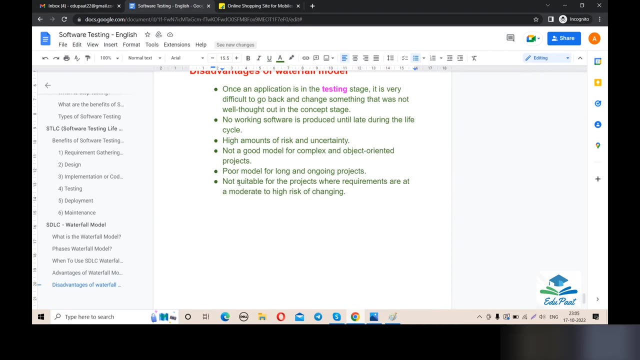 i will discuss on the later video. then poor model for a long and ongoing projects- as of guys have already discussed all these things- and then not suitable for the projects where requirements are not a moderate or too high risk or changing. if there is frequent changes of project requirement, then this waterfall. 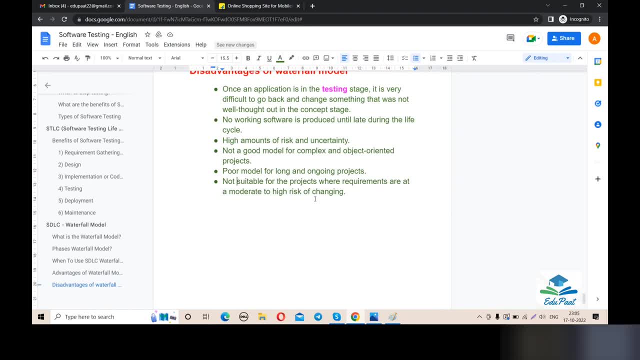 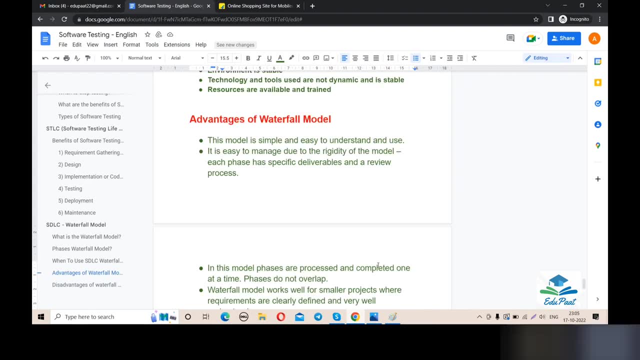 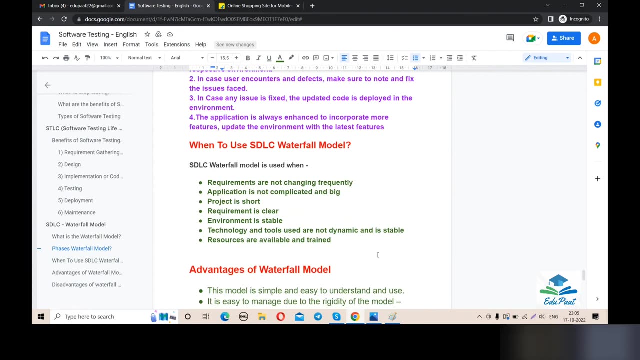 model is not the suitable right. so that is the disadvantage of waterfall model. okay, so now you guys are very clear about what is the sdlc waterfall model, what are the phases of that, what is the advantage, what is the disadvantage when we use, when we use the sdlc waterfall model. so if you